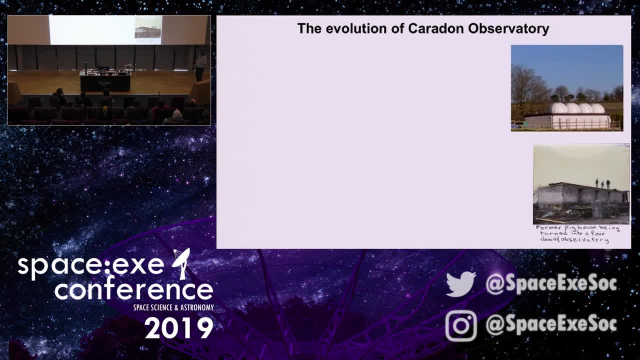 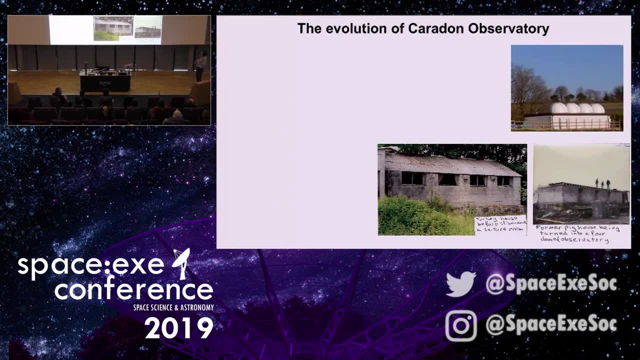 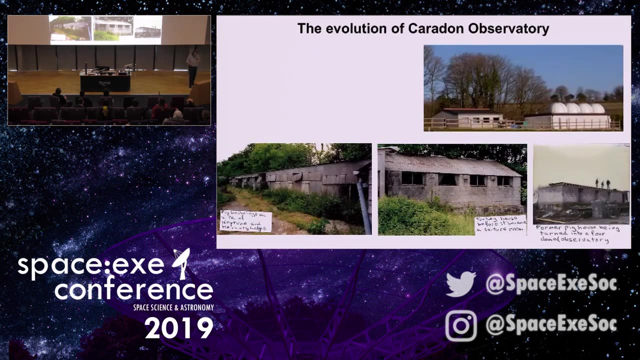 we could talk to people who were interested in there, which we called the lecture theatre, which started out as the turkey house and it somewhat evolved to that, And then we had the row of pig buildings And we thought that's probably not entirely satisfactory. 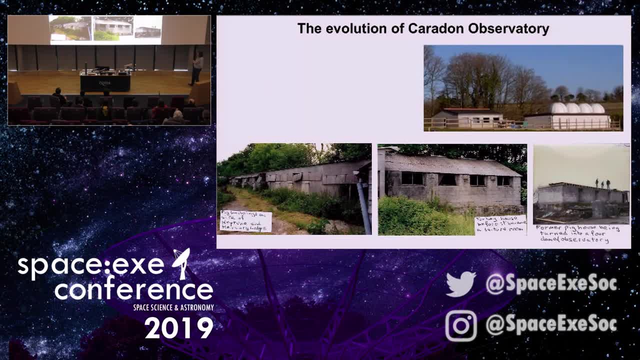 for astronomers to come and see it. We thought we would go and take a look at the houses And we had a guys who were there and look at the houses and they were actually three to stay there. So those are our accommodation lodges. 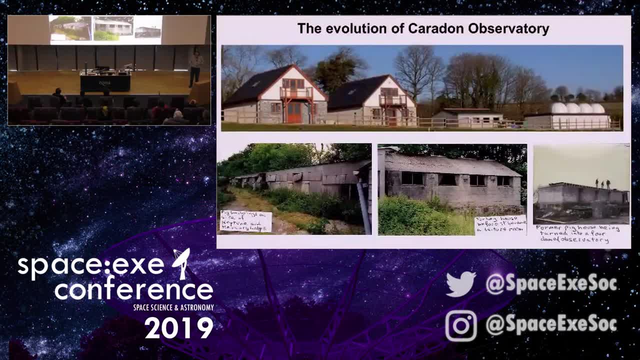 So that's basically what we've got at Carradine Observatory: Our motto, our mission statement. when we started out doing this, we'd seen other mission statements and they seemed to be long and complicated and a bit cheesy, So we got a very simple one. 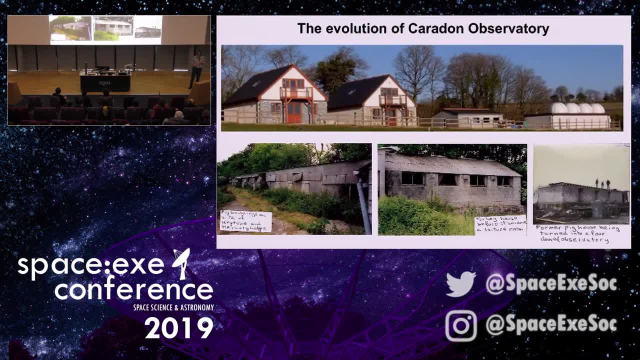 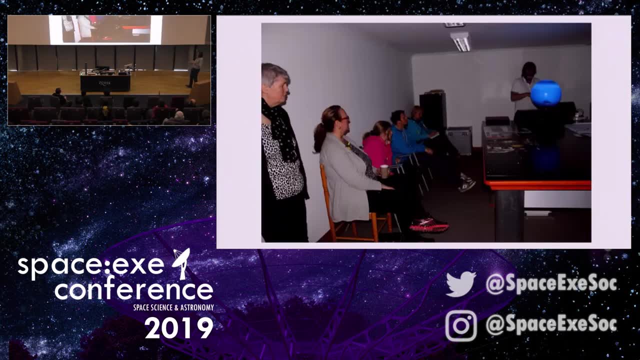 Our mission statement is: why not? So if somebody says why do you do astronomy, Say why not? We'd always try to do the best that we possibly can. So there's inside the Turkey. I'm sorry, there's inside the lecture theater. 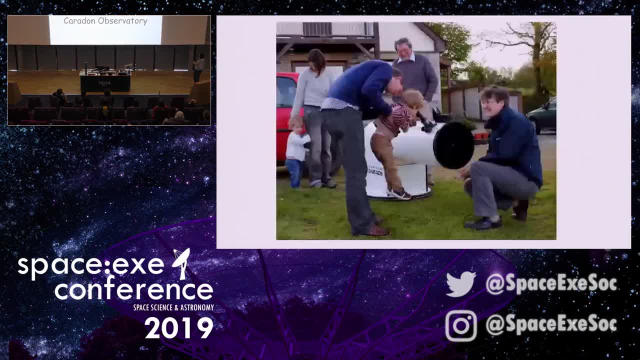 and I'm using something called Magic Planet there And we've also got- sorry, I'm not very good at using this better- And we have open days where people come to find out, to just outreach to people, start them young. 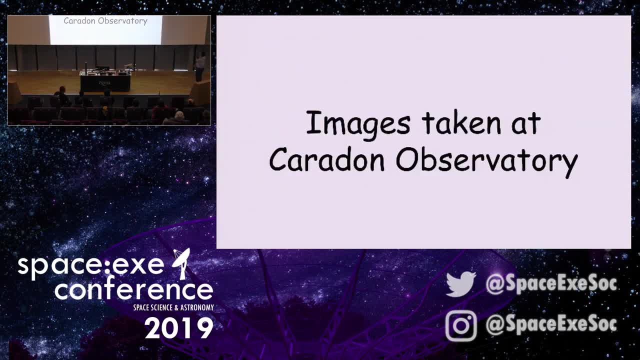 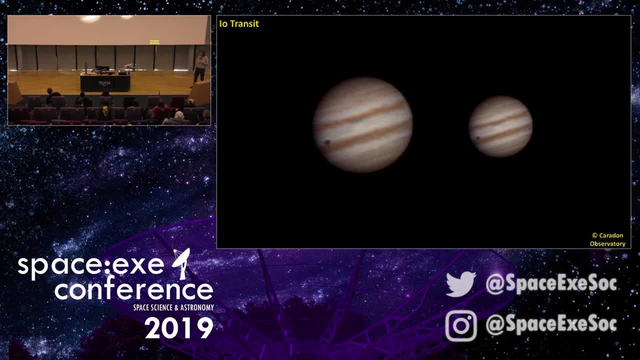 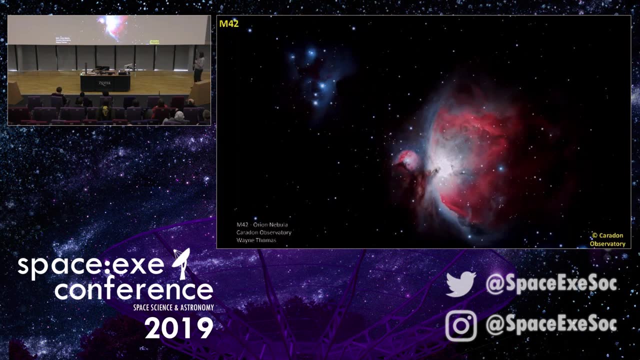 try to encourage them. We also try to work as hard as we can to get as good images as possible. So there's a transit of Io passed across in front of Jupiter. There's M42, the Orion Nebula. we'll come back to that in a little while. 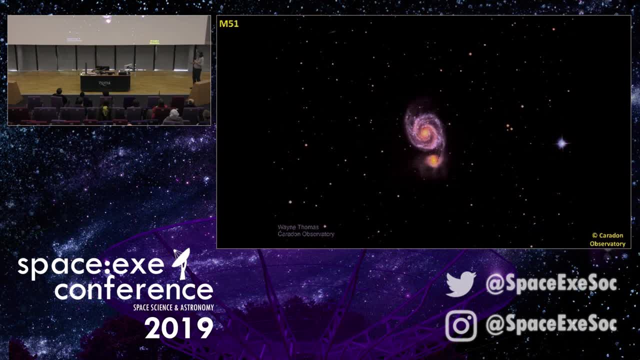 There's a shot of M51, that's Wayne Thomas, our principal observer astrophotographer. We also tie in with people doing GCSE astronomy And that was one of the images that was requested by one of our students as part of their coursework. 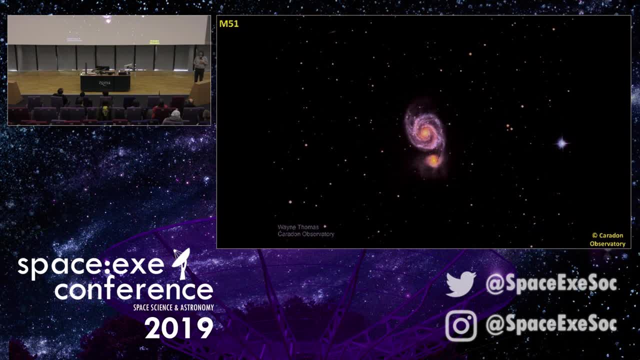 We have to make sure, when we're doing that, that we do exactly as they specify, because part of their remit is to say so, how are you going to improve on it? So we thought, if we did something that takes five hours, and then say to them: 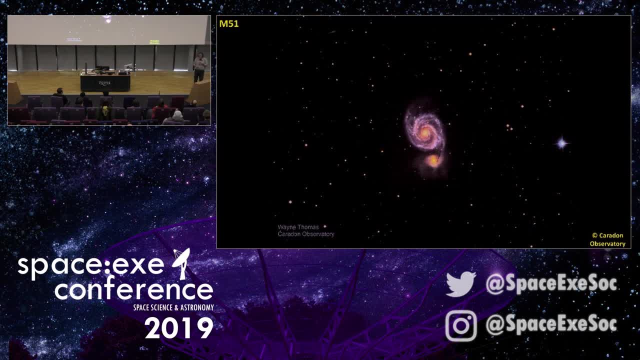 and we might be dealing with 13 or 14 year olds right. go and hit the library for the next fortnight to see if you can work out how to improve on that. So it's one of the things we have to be aware of. 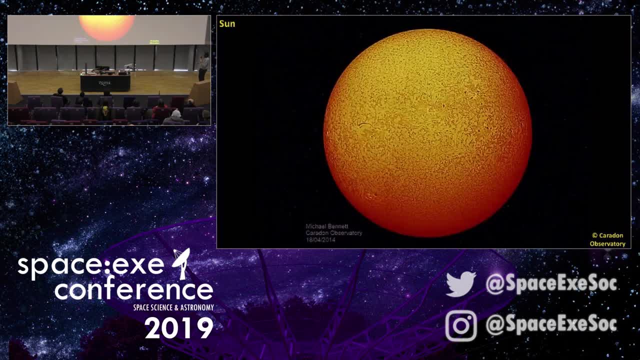 There's Bode's galaxy And there's through our solar telescope taking an image of the sun. So what I've tried to do there is just give an idea of the sort of things that we try to encourage, that we do ourselves. 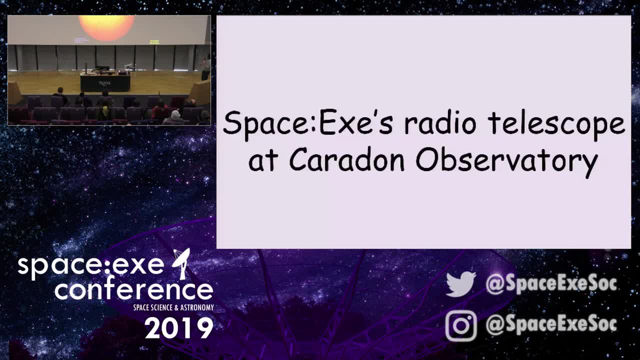 we try to encourage other people to get involved in, And one of the things that, when SpaceX said we are trying to find a site to locate the radio telescope, would you like to get involved? Our mission statement was: why not? And so we did. 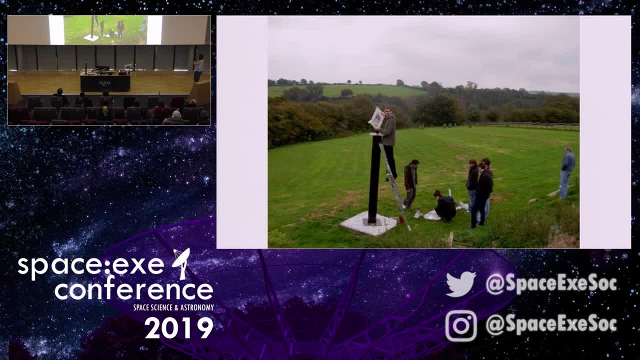 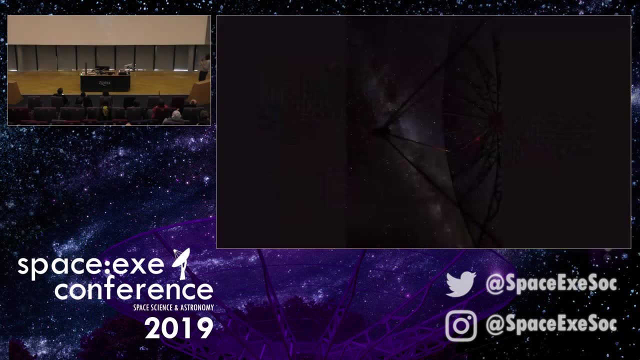 So there it is to start off with. Base has been put in, There's the central plinth And there we build it up And sorry, I don't know if you can see the lights there, but that's a shot trying to show. 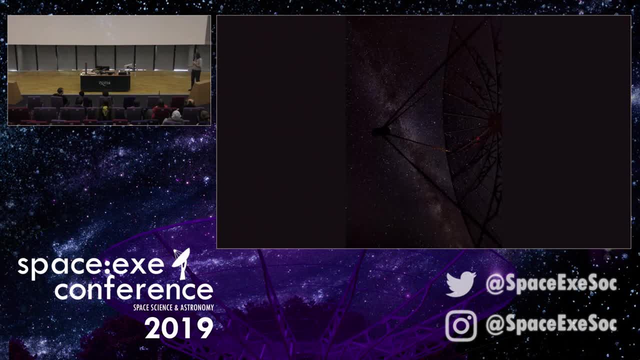 there's the radio telescope pointing up towards the heavens. Do you want to go back? We can turn the lights off for a sec. Yes, okay, That's much better. That actually shows, in fact, what I'll do is, if it's all right with people. 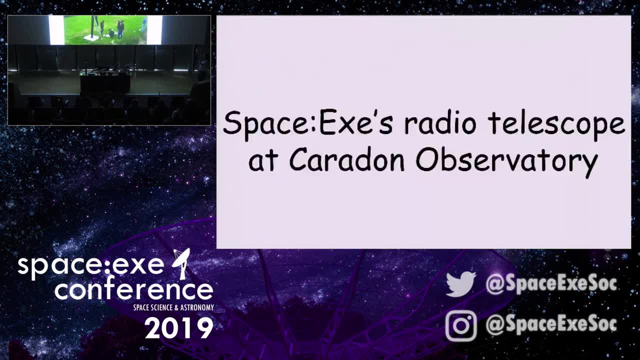 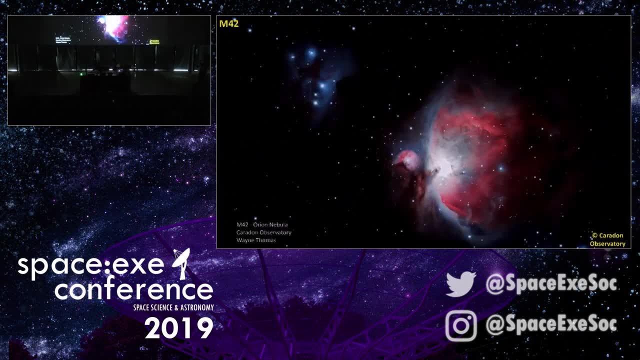 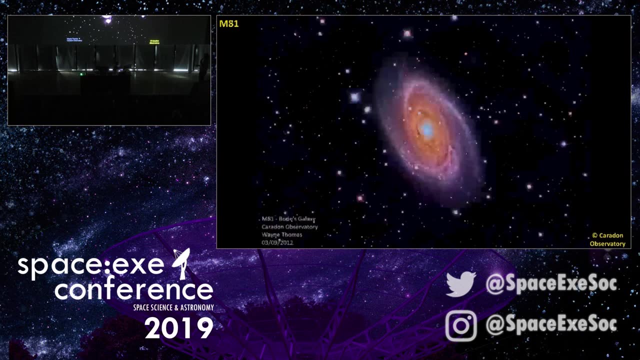 I'll just run back just a little bit so you can see some of the other pictures that we've got. But there's M51, there's the Orion Nebula And, if I'm gentle enough on this, Yep, there's Bode's galaxy. 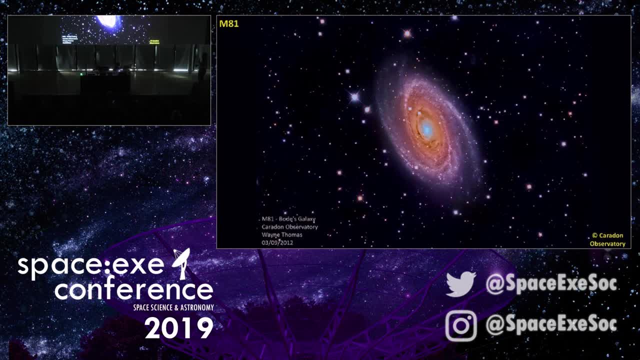 It's about 12 million light years away. Kids find this fascinating when they come to look at it. My best way of saying it: if you've ever been to a reservoir, driven there in a car and they say: well, yes, because we've got a local one. 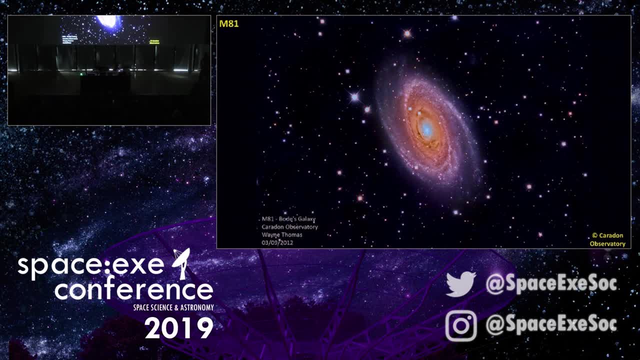 Sibley Back and say, well, when you're looking at Sibley Back, there's probably some raindrops on your window screen, on the window of the car, So most of the things in there are the equivalent of the raindrops on the window. 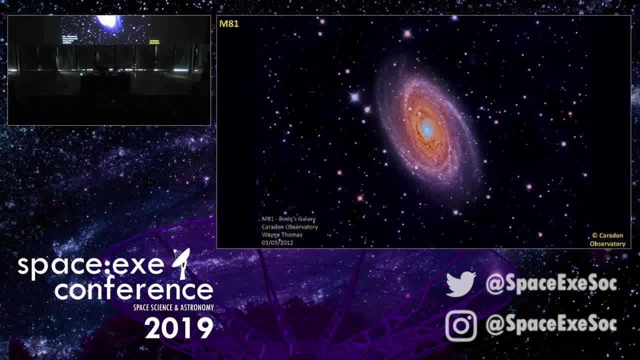 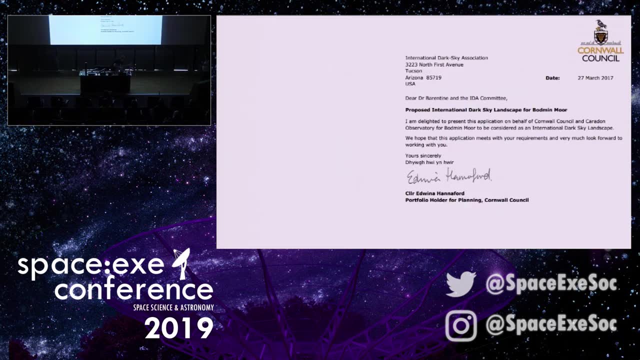 and far beyond is a huge collection which is an external galaxy, So let's take this through as far as there. But one of the outreach projects that we got involved in was with dark skies. We had come for a long time to realize. 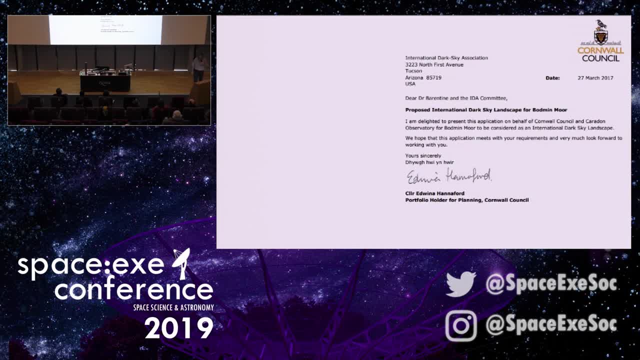 that the skies over Cornwall were exceptional and that we should try and find a way of getting this recognized. So we got in touch with the International Dark Skies Association to find out how could we actually get this area of Bodmin Moor, because we are on the extreme edge of Bodmin Moor. 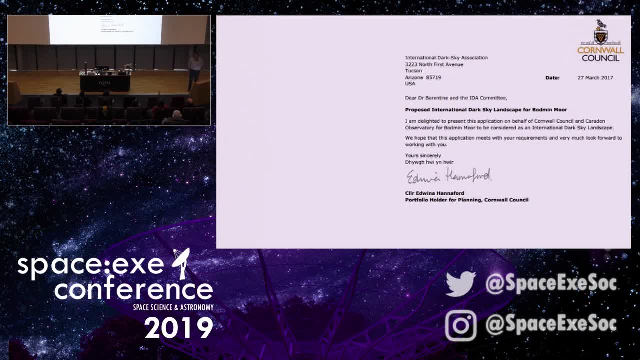 was there any way in which you could get a dark skies designation? Well, CECF kind of signed me And they said yes, but unfortunately, with the sort of thing you're looking for, you are not a big enough entity. What you need to do is to get minimum size of it. 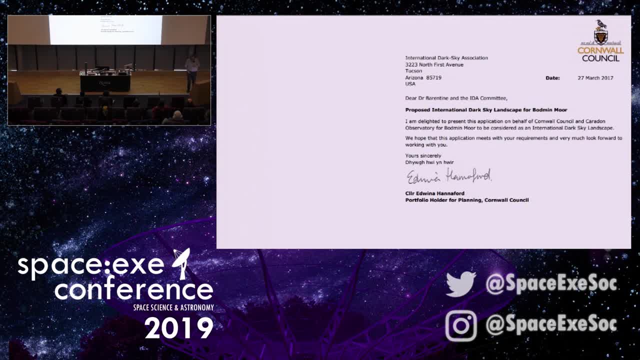 would be your county council to get involved. So we stopped getting involved with the Dark Skies Association and got involved with Cornwall Council and guided and enthused them until eventually they were prepared to say, yes, we will form a collaboration, but unfortunately it isn't going to happen. 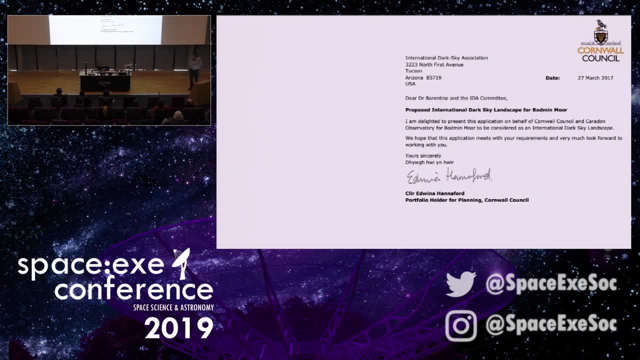 because sadly we don't have any more time left. It's the community that needs to come forward and we need to with you, and we will go to the dark skies association in tucson in arizona and we want to get designation of the dark skies park for bob min more, and i wish i was more delicate on doing. 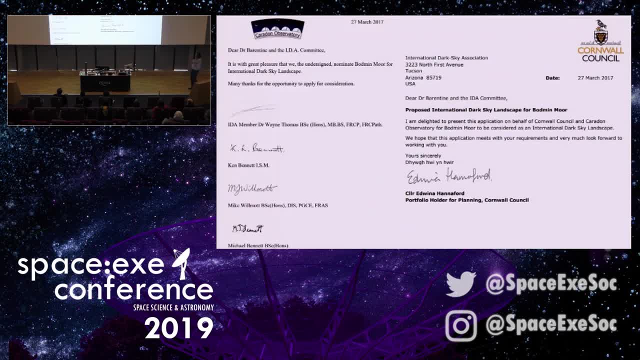 this. okay. so there's a cut down letter. i don't want you to give the impression that that's all that you send off. that's just saying there's the council's letter and there's the start and the end of our letter, with the various directors on there signing it off. um, just to give you an impression. 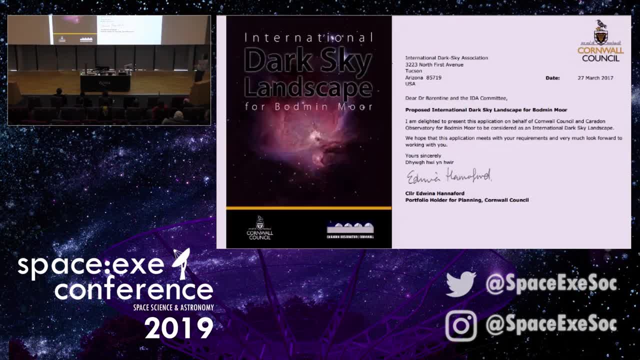 that's not all you said. and in that dark skies landscape and there's something interesting when we, when we were trying to get involved with doing this, there were a number of things where they came back and said: we want this checked, we want this checked, we want this checked, and we thought we 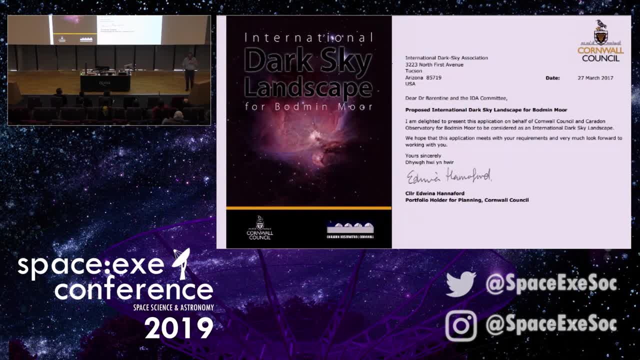 ticked every box and then they came back to us and said, uh, there's been a slight delay and so you think you know whatever's up now, what's the next delay? we thought we got this all signed, but it was a rather nice delay. they said we've just realized that you are a site of outstanding. 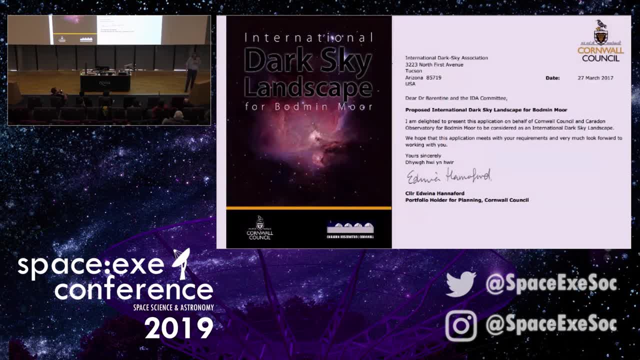 natural beauty, and you're also a site of special scientific interest, and you're the first one in the world who's actually put forward for dark sky status for something that already has those two statuses already. so our committee has decided that we want to create a brand new designation. 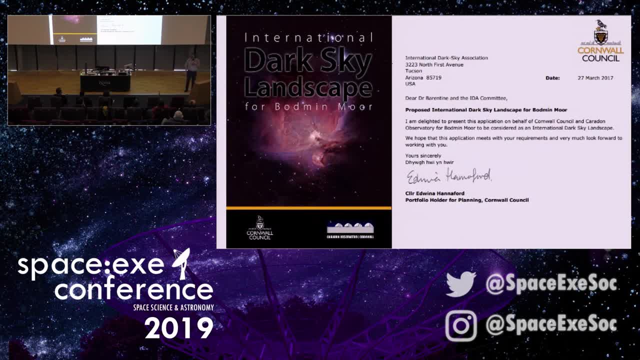 and we're trying to find what is the appropriate name that you can, that we can do. so they got back to us and said: will you please resubmit and we'd like you to call it a dark skies landscape, and Bob Minmore is actually the first. 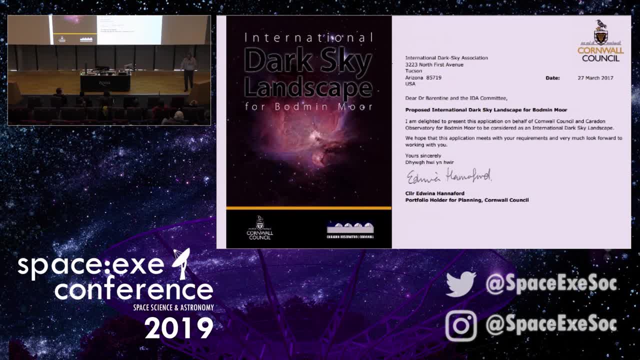 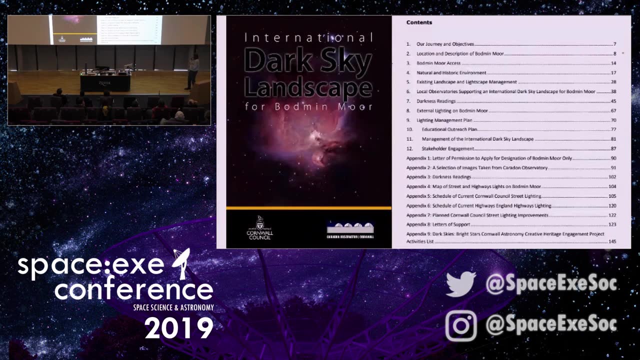 dark skies, landscape in the world and we have set a precedent- which means other areas now that have got special scientific interest or particularly beautiful places. about the precedent created with Bob Minmore I said to you before you don't just include that letter, that's actually the letter. 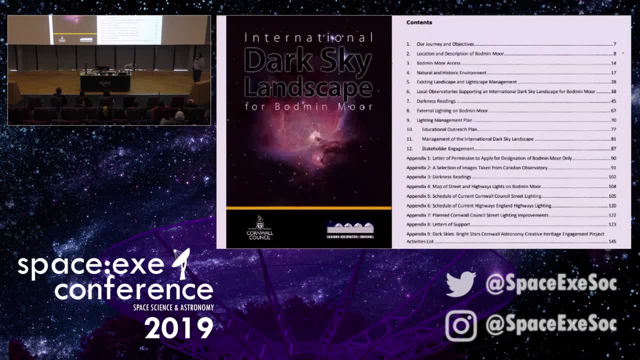 that went in. it was 145 pages long and it's a pretty, pretty complete document. thing is you have to identify. you don't just say I want to be one of those and say, great, you've got it. now what are you going to do to keep it going so? 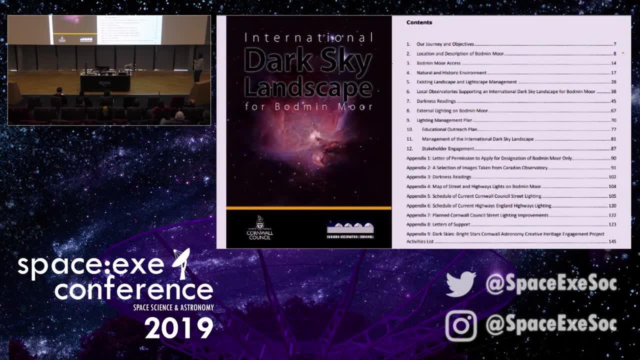 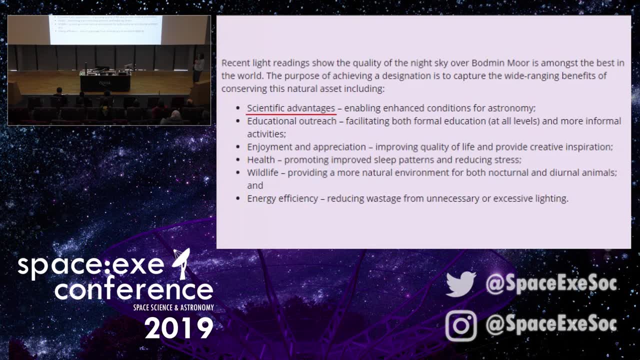 we had to have a rolling program to keep it going. those were some of the ones that we thought were interesting and of advantage. the scientific advantages, education, enjoyment, health, wildlife and energy efficiency- all those were included and what's good about this is they don't say everybody's got to have their light shielded, go back and change everything but what the council. 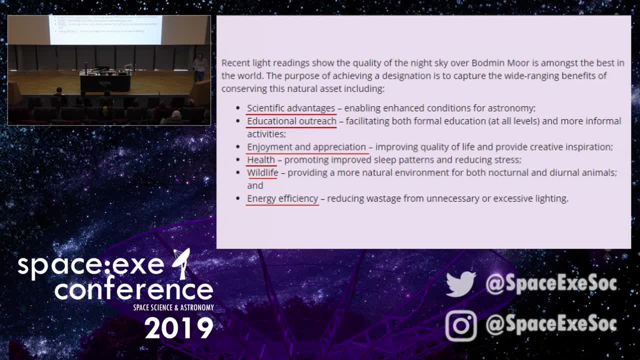 has agreed in Cornwall. I'm sorry if there's any questions, if there's any questions, if there's any one in Cornwall from here who's going to get caught by this. but in Cornwall now you put in an application for upgrading your lighting or you ask for new lighting and you've got to conform to. 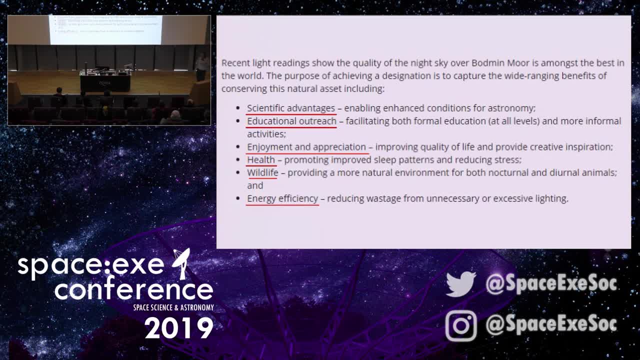 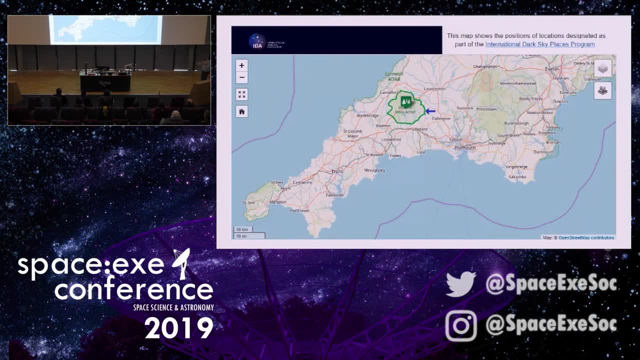 to the new things that apply across the whole of Bob Minmore. okay, so where are we? well, there's, that's the area that's covered. there's Bob Min. there's, there's a Carradine Observatory right on the corner there, and so we coordinate and work with the council on that. and, for those of you, 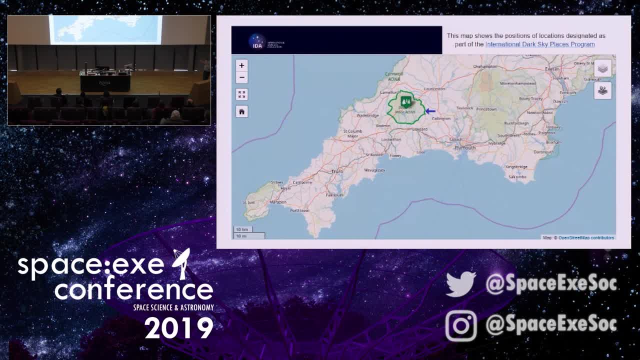 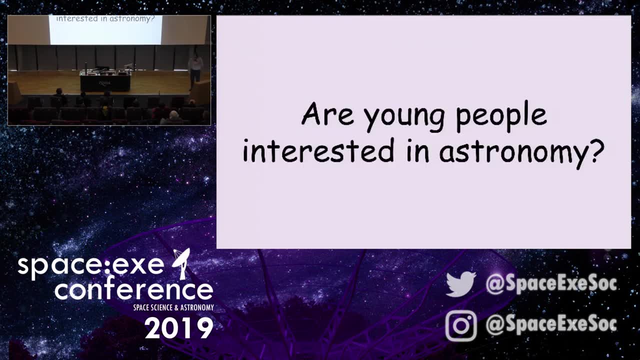 interested from here. you can get to it either by going down the A30 or you can go down the A38, and that includes our friends from Sidmouth. so if you want to come down anytime, please do. okay, that was setting a bit of what we've done at the moment, of why we, why we've done it, why have. 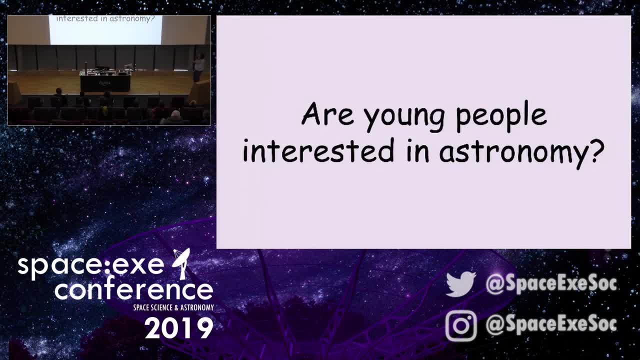 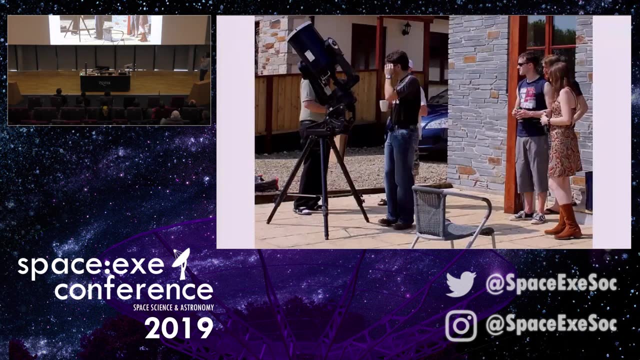 we created this infrastructure. well, we're really we're trying to answer the question, or we know what the answer is, but we're trying to provide evidence for the fact. our people, our young people, interested in astronomy and the answer is: you bet they are um, these are carried an observatory where we had one of our opening days and we have people come. 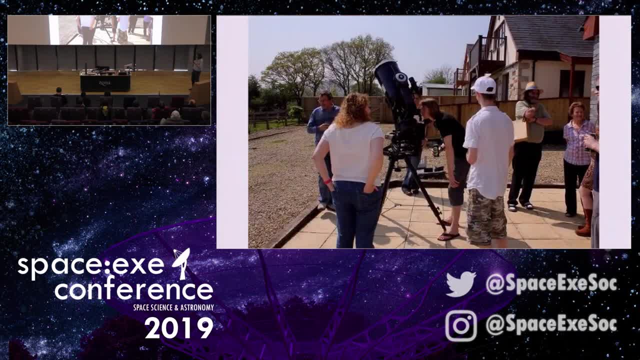 in. obviously, during the day we can have to operate the solar telescope. this is not the sort of standard one where they say I've got this- uh, very cheap telescope and this tiny little solar filter that you put on the IPS end, which are worse than useless. they're more dangerous than you can. 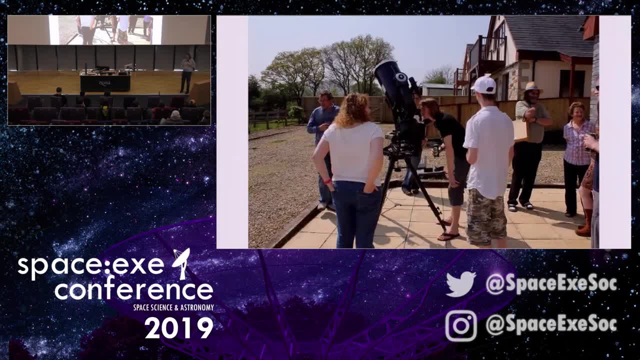 imagine. I think the best place for those- perhaps Patrick Moore once said the best place for one of- is at the bottom of the fish tank. It might interest the fish and it will certainly deter you from trying to use it. So what we have got is we have got the proper Mylar filters. 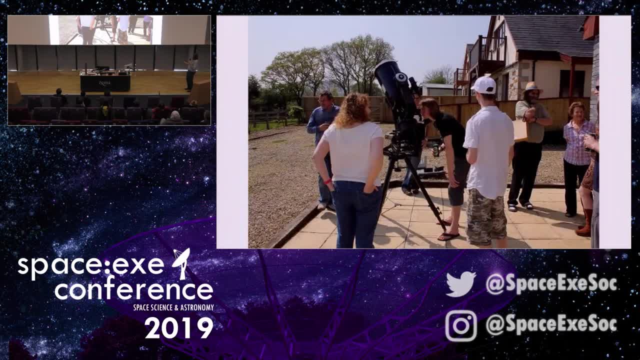 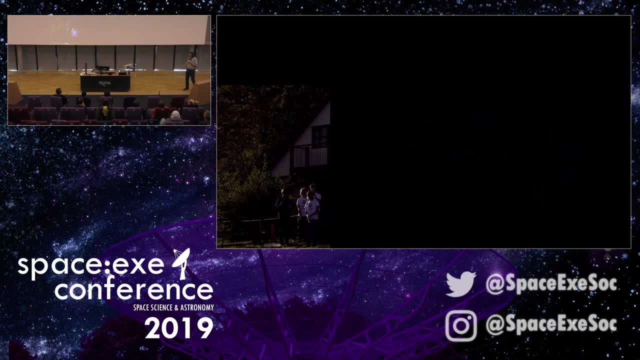 on the top end of this, restricting the light that comes in, not trying to compensate with the concentrated light that's coming out at the other end. Sam, can we have the lights down please? on this? You mentioned about rockets. We sometimes run various sessions. 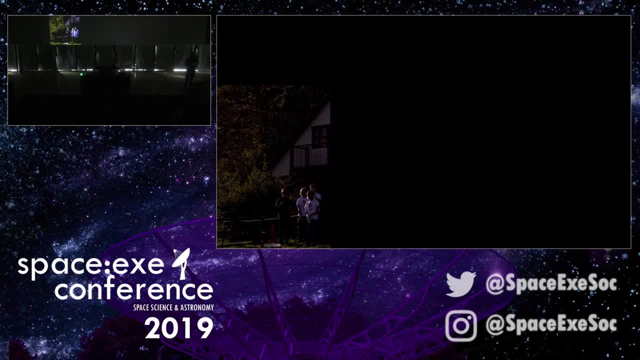 where we deal with rockets We had to also coordinate with the local fire brigade, etc. But it was rather nice that we had some youngsters who came out there, worked on a project with us and it's perhaps not terribly clear over there what's going on. 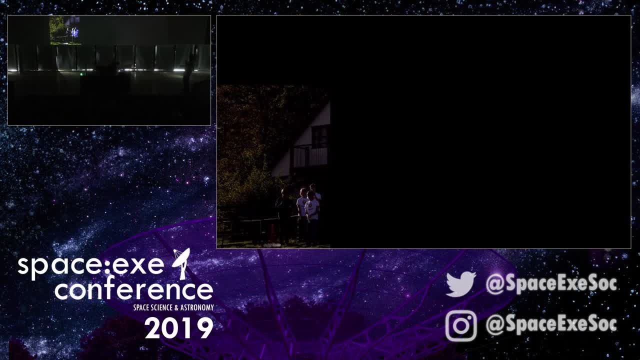 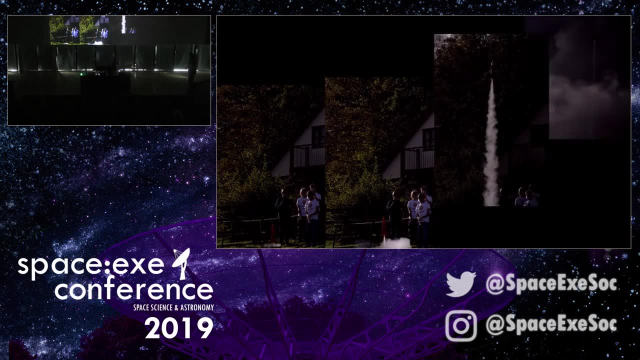 but if I manage to get on to the next one, they've actually designed and are building a rocket which is taking off there And, yes, we did have a parachute on there. We didn't get it back immediately, but about two days later. 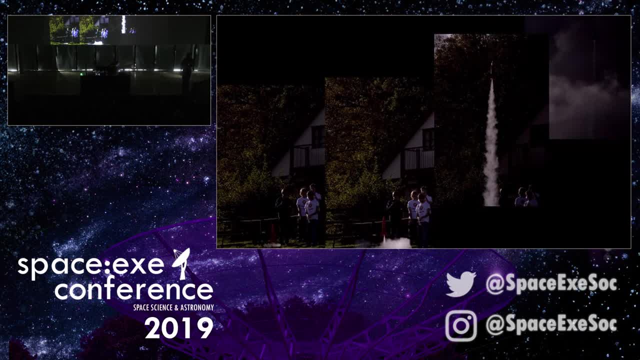 the farmer from Three Farms Across said: is this anything to do with you? because it arrived in my yard three days ago when I was trying to work out who would be weird enough to do that. He said So. he said so it's just taken me. 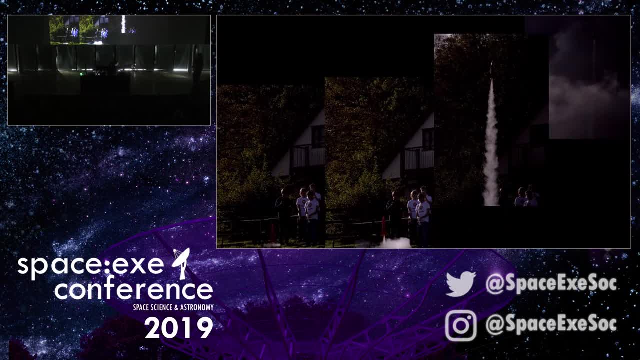 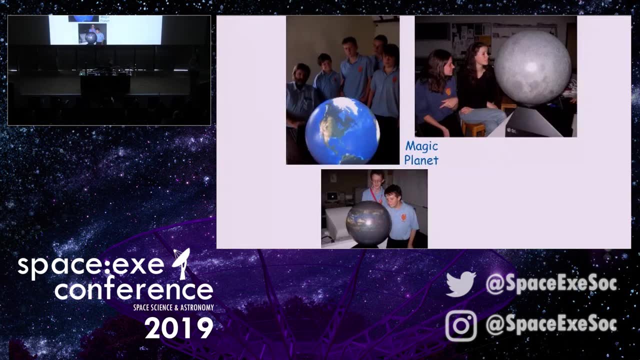 He said I was busy for the last couple of days, but I knew where I had to come and do it, because if it wasn't you lot, you'd know where it was OK, We've also got something called Magic Planet. This is quite an amazing device. 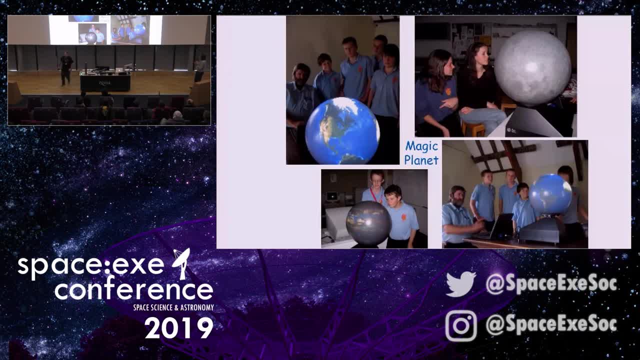 It represents something. Just checking time here. One of the biggest problems that we have when you're educating children is they see a world map. They've seen loads of world map. They're in books, they're on the web, they're up on the wall. 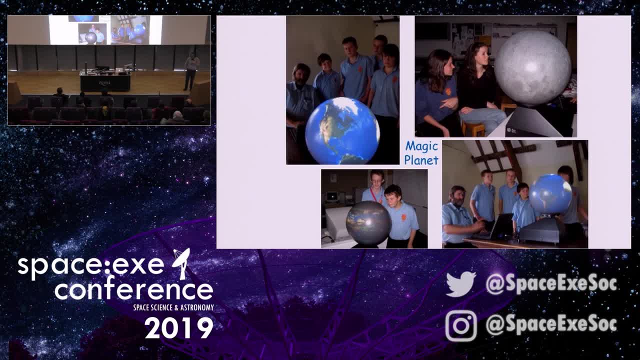 Most children, by the time they get to secondary school, know exactly what the world map looks like. They know exactly where they are. They can recognise the world on which they live. Biggest problem, of course, is that there is no world map. 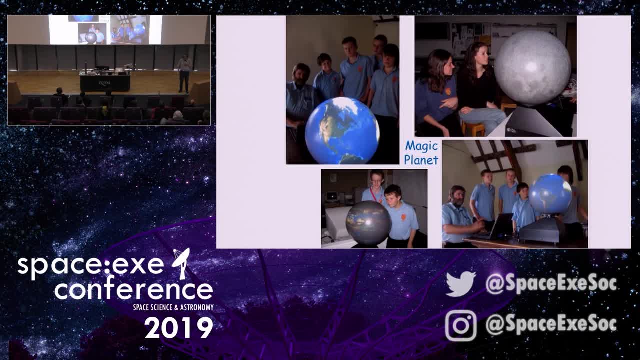 that has yet been created, which is not hugely distorted. In fact, the only thing that's accurate on a world map is is the equator line. Everything else is wrong, and the further away you go from the equator line. 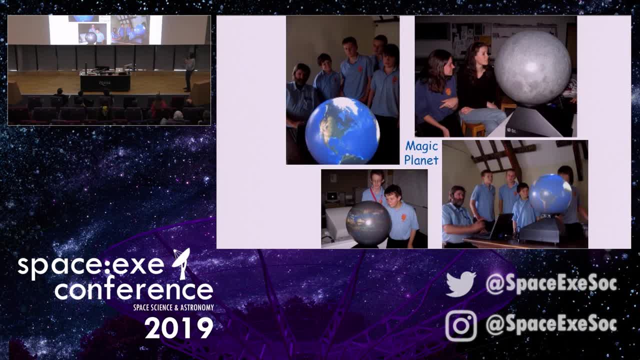 the worse it gets. So what we rather like about this is that we can create. We use some specialist software that was written by Global Imaginations in California. They have worked with NASA, who have got a briefing which says: everything that we find out is owned by the American taxpayer. 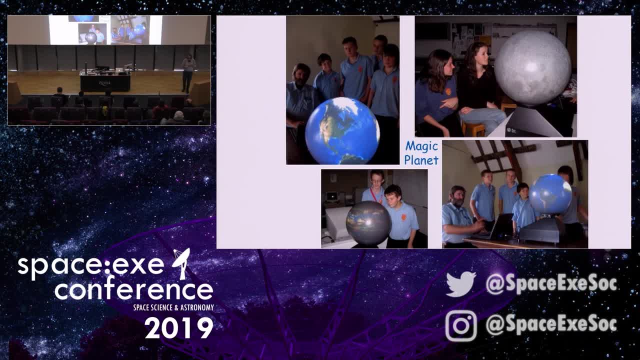 We will publish everything that we can in as many different formats as we can, and Global Imaginations came along and said we can create a spherical surface. How about you give us all the close-up images that you've got from your planets? We will actually create undiscorted pictures. 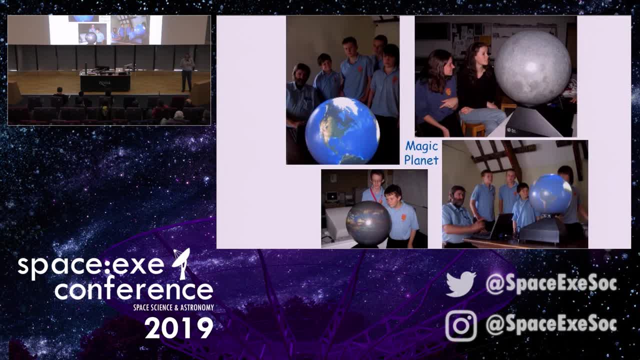 of what all the planetary surfaces look like and the major moons, and this is what we've got Now. I think that's fascinating. but I think what's also interesting on there is how interested the kids are there. These are not posed just to give you some idea. 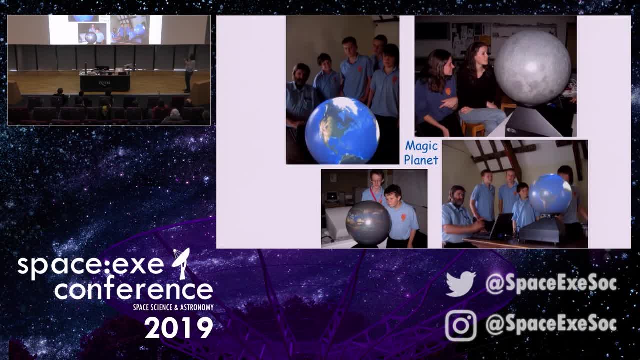 about what I'm talking about. These are all GCSE astronomy. These are all GCSE astronomy. These are all GCSE astronomy. students Most of you know GCSE is done in year 11, under normal circumstances, but not with the way we do GCSE astronomy. 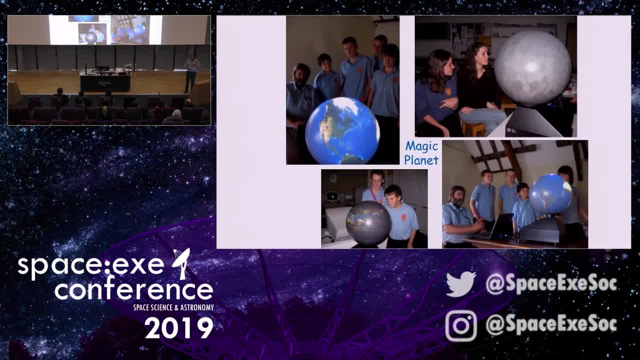 The kids start it in year 7, and they can take it when they like. I've had no children so far who have opted to take it in the end of year 7, because they normally ask me a question: can I take it in year 7?? 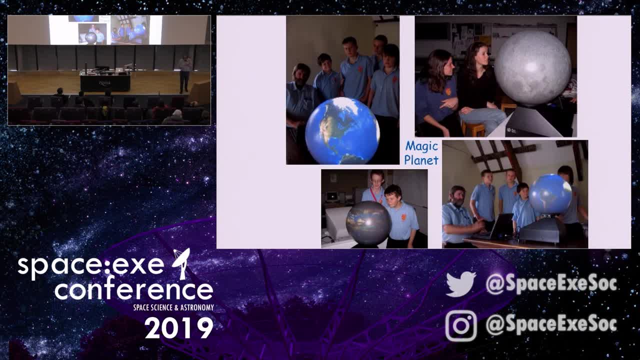 And I say yes. And they say, if we do an extra year, will I do better? And I say yes because I think it takes a couple of years to really get to there. You want to see the spring on the step it takes. 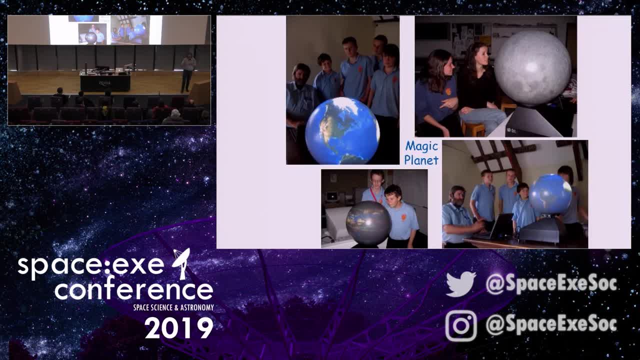 when you've got a kid going into year 9 who has just taken a full GCSE in astronomy in their back pocket already I speak to other teachers and say we can tell the astronomy students they come in to start their GCSE with such confidence. 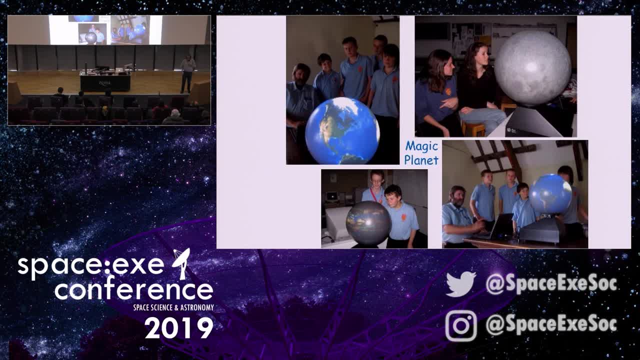 Unlike others who are saying: can I do this? The general approach for the successful astronomers is saying: is there any reason why I can't do this? And it does make a difference. Just to give you some idea, these two lads here, Alex and Barney: 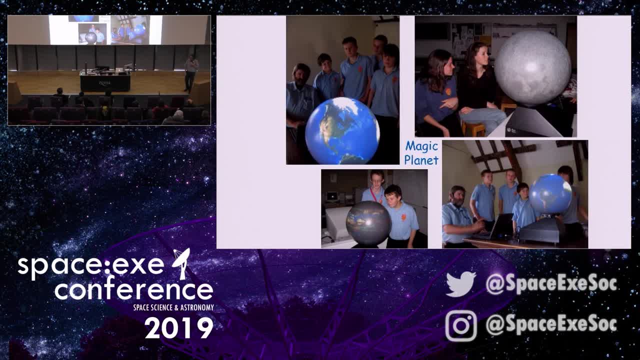 they actually did their GCSE in year 9.. They said, well, you want to stop now. What can we do? Can we do A-level? I said there is no A-level. I said the only thing there is. 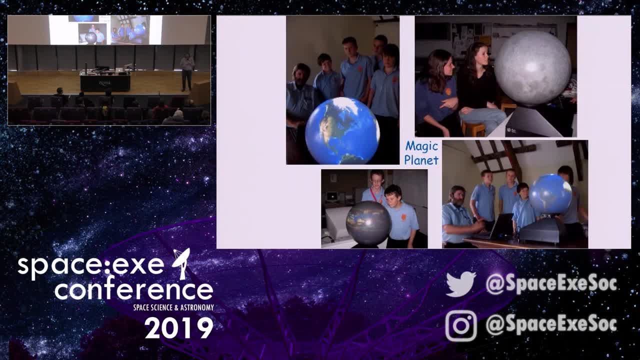 there is a cosmology module in A-level physics. They said, great, Can we do the cosmology module in A-level physics? So I said, yes, you do realise that it's only part of an A-level and you won't get the rest of the A-level as well. 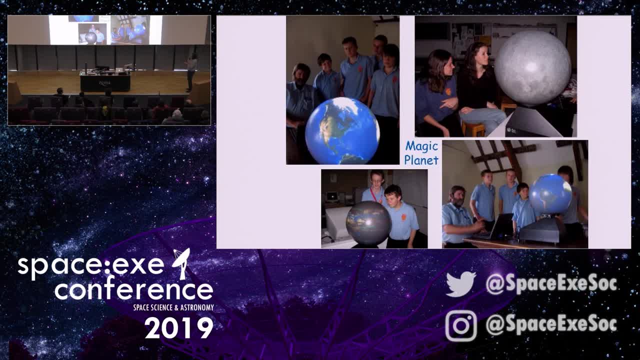 I said: we don't care, We just want to do it for fun. So we had two year 10 lads here who did a year 13 cosmology, cosmology module, which they passed. They failed the A-level physics because they didn't do any other modules. 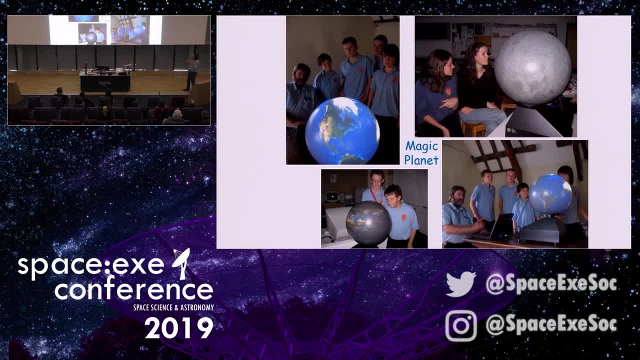 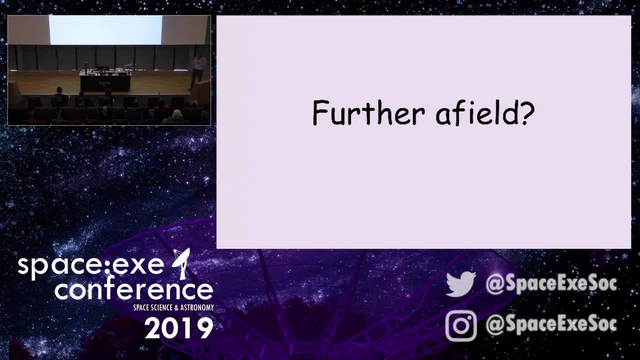 and they were entirely happy with it. We got kids who are so wound up with astronomy. they really love it. They really do Okay, anything further afield? Well, that's the ING, the Isaac Newton Group of Telescopes in La Palma. 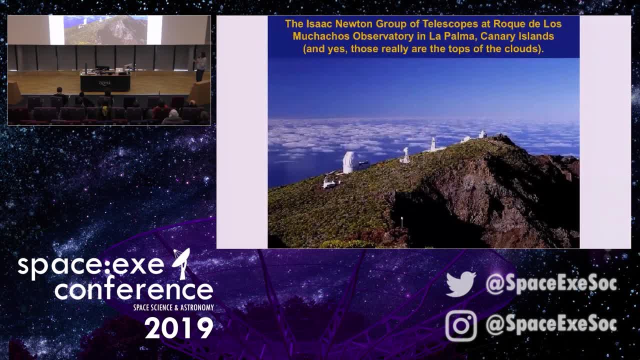 the Canary Isles And as you look across the sea, please note that that is not the sea. That's the top of the clouds. Now, back in 2000,, I had some kids, because before I was teaching astronomy in Liscard School. 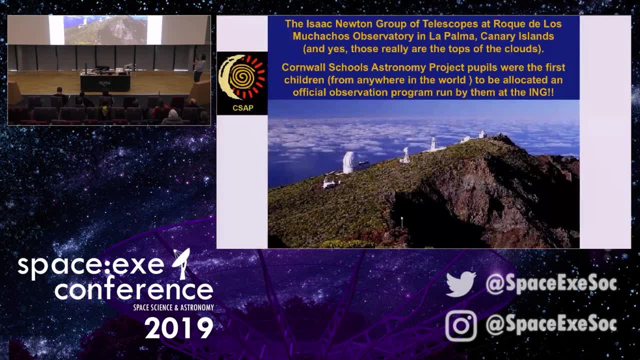 which is where I teach GCSE astronomy. I was actually part of the Cornwall School's astronomy project, which two other teachers and me set this thing up, and we got an invite to- what about taking some children down here? Because we'd liaised with this on a separate. 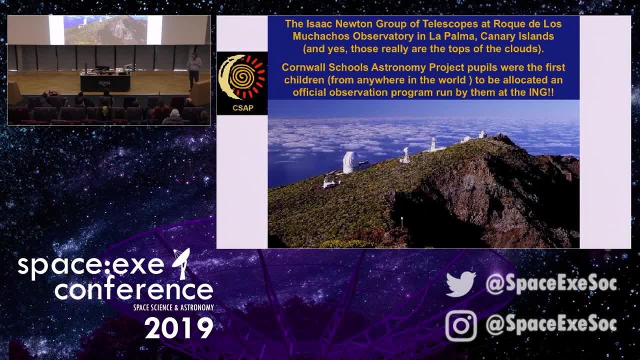 but with them on a separate project. And they said: what are you doing with these kids? They are very young and they seem to know an awful lot. What about bringing? do you want to bring some kids down here? We could see if we can get some time for you. 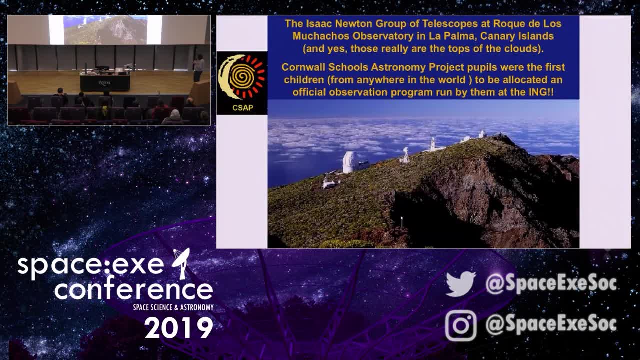 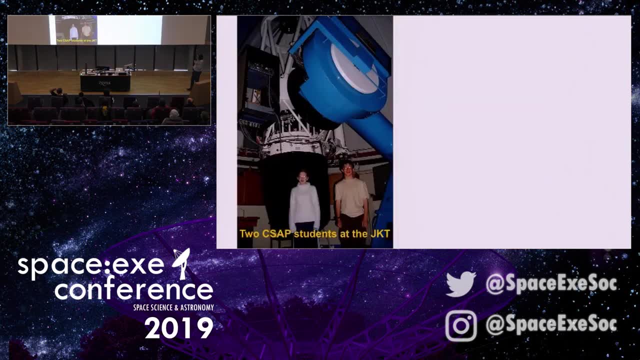 I said, yeah, we would actually love to do this. So we actually worked on. that's the Jacobus-Captain Telescope up there and that's the one that we worked on. So there are a couple of our students working on the Jacobus-Captain Telescope. 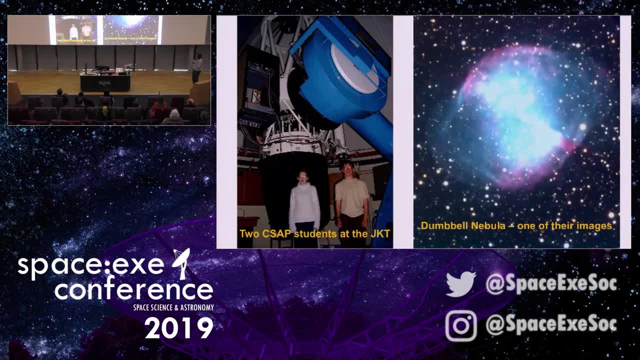 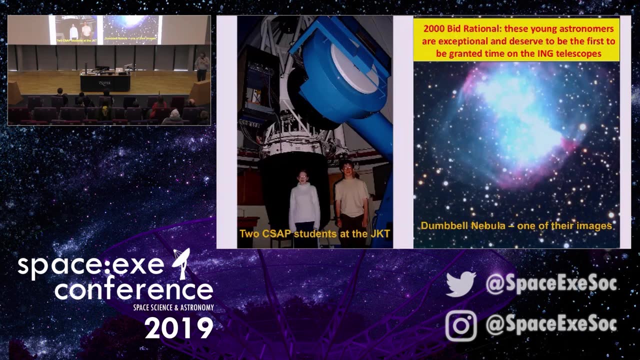 There's one of the images that they produced. They were both 13 years old at that stage And the rationale? the rationale was: there are some exceptional astronomers here. What about being the first in the world to offer them telescope time? Funnily enough, just checking time, yes. 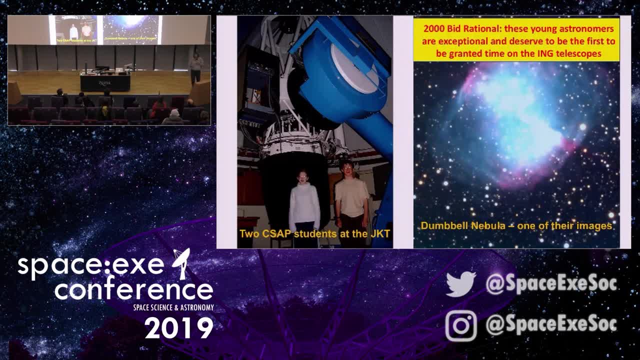 Funnily enough, when they came back to us and said: look, we're terribly sorry. We've just checked our charter. We have got absolutely no facilities for children at all, So we can't do it. I'm terribly sorry. 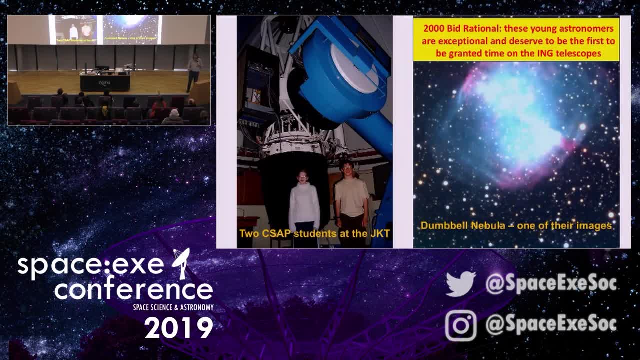 And I said that's a real, real shame because the kids would love to do that. They said we would love to do it, But I mean the only way we could do it. would they be happy if they had the status? 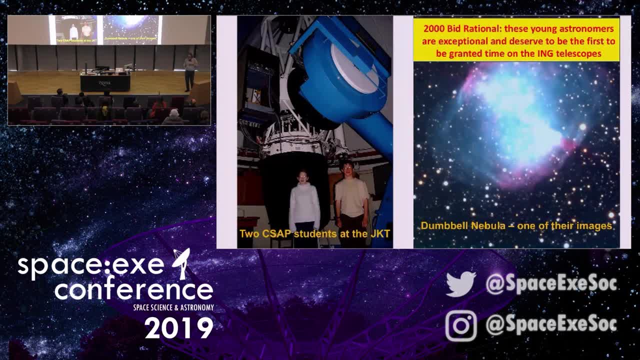 of visiting an astronomer. So I spoke to the kids and said: how would you feel about going to visit this place as a visiting astronomer? And they thought about it for getting on for a tenth of a second and said yeah, yes, please. 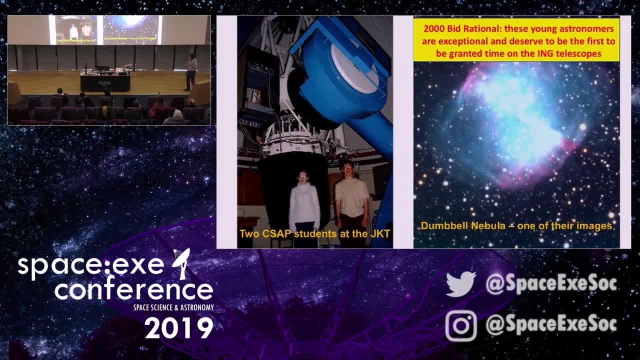 So we went down there. So that was what we did in 2000.. The following year, of course, we couldn't do this again- You can't be first for a second year- So we had to try and find a different way. 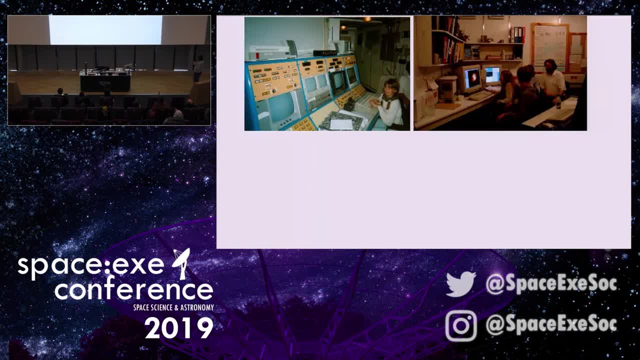 and wanted to take them down, And so there they are again. All right, so we've got some of them there working. And, funny enough, when I mentioned this to Sam, Sam said: I recognize that control bank because I've been down working at the IMG. 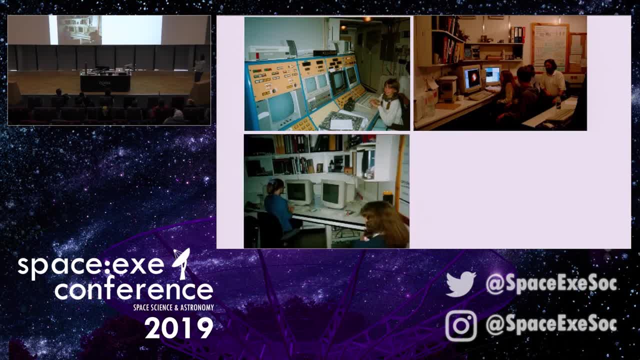 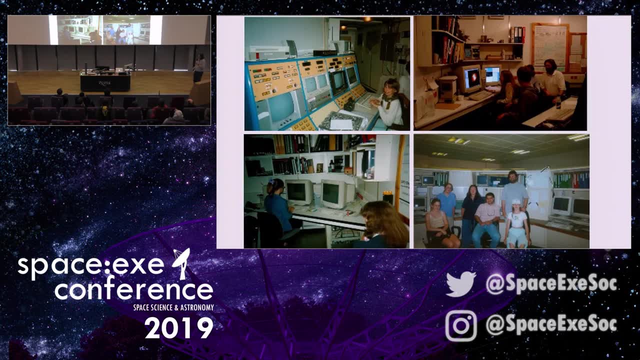 So that is for real. And there we are, And I'm afraid that one there, I'm afraid there's me looking somewhat younger than I am now, probably a little less Harris, But there they are, And the rationale that we used was the next generation of astronomers. 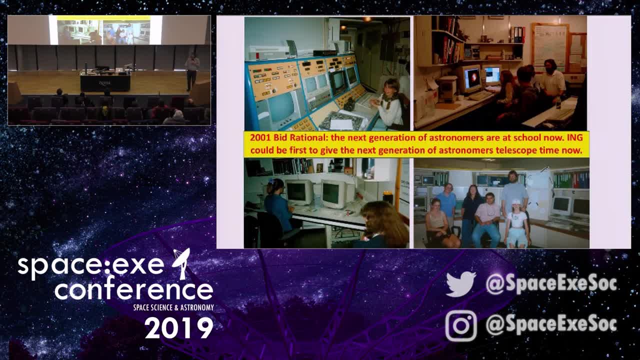 are at school now, So would you like to be the first in the world to allow the next generation of astronomers to come and work on your telescopes? And they said, based on last year, yeah, we will have you down. They were brilliant, these kids were. 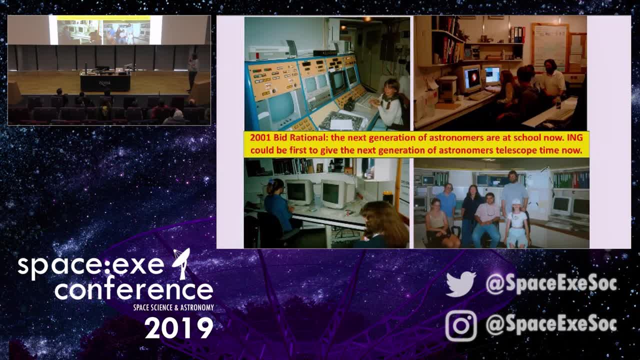 They were absolutely fantastic, And I say that because partway through they had an emergency project came through. Whenever you get booked telescope time, you have to allow for the fact that there could be an hour or an hour and a half when an emergency project comes through. 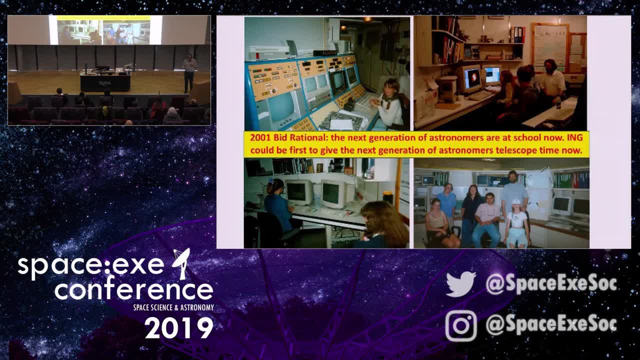 And it just so happened on the night when we were there that happened. So my kids, who had already impressed the ING staff because the first day you learn the computer programs- Now I don't know if how many of you are familiar- 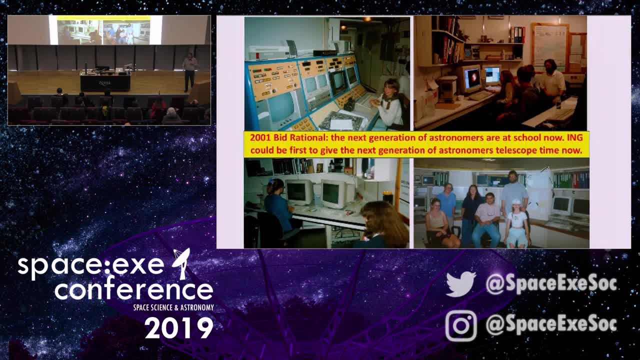 with just how quickly kids devour IT understanding. So we went through the first day And after an hour and a half the kids were fully aware of how to operate all the systems. And the guy who was there- our contact there- called Javier. 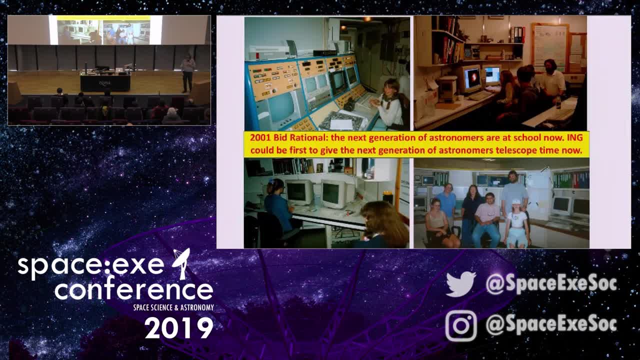 he said: we've never had anybody Pick up these systems this fast. Astronomers normally take all day to understand what's going on. How's this happening? I said: have you ever had any kids here learning to use IT before? 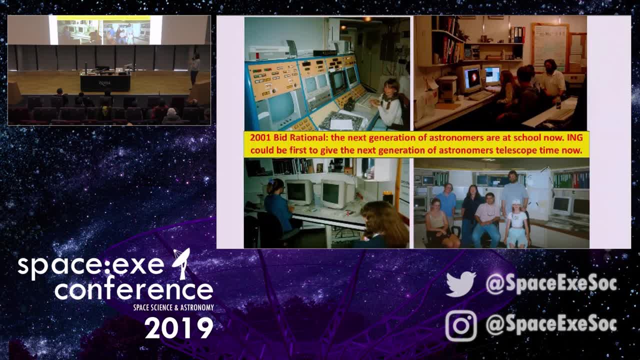 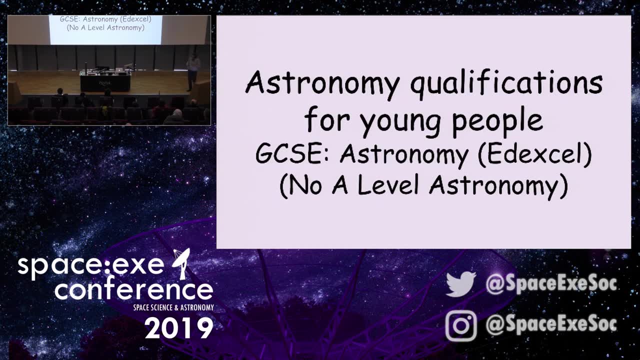 And he said no. He said, well, you have now. So that's where we were with that one. One thing that I've mentioned- and it's true, is that astronomy qualifications for young people. there's only a GCSE in astronomy. 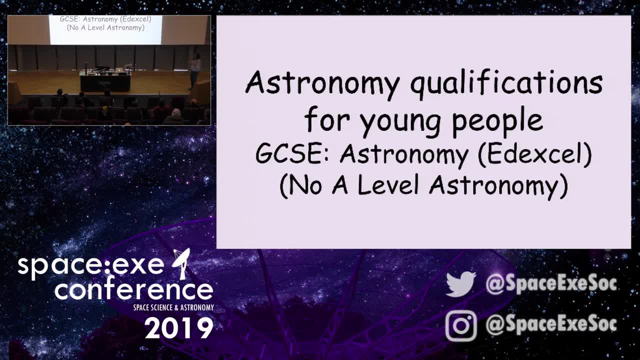 It's only run by one exam board. I wish it was done by more. and there's no A-level astronomy, And I wish there was, because there are enough kids who are interested in doing this. So where are we at? I said you've got to look at the past. 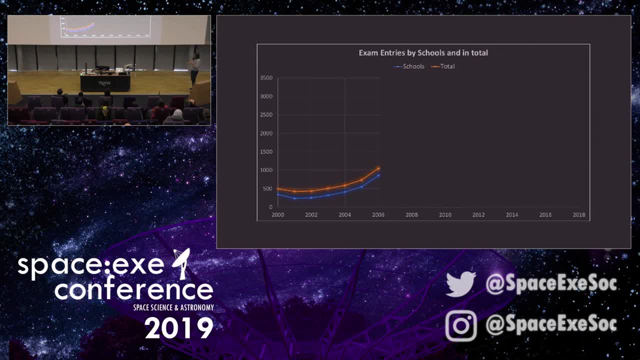 see where you are now to work out where you're going to go in the future. Well, that's when we started And what I've listed there is the total number of candidates who are taking the exams, plus, in blue, the number from schools. 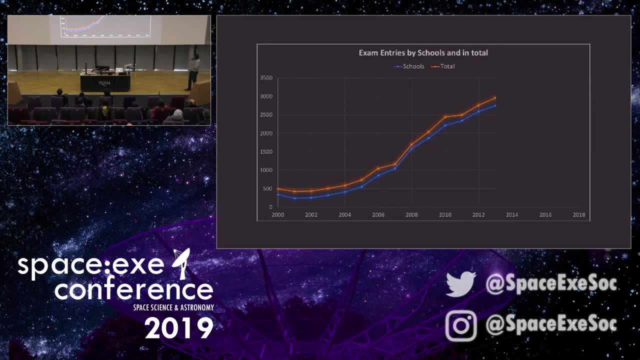 So at the start it was looking pretty good. It then shot up to about 2013.. Things are looking really good there. It's up by a factor of well. in 2002, it was below 500.. And we're now close up to 3,000.. 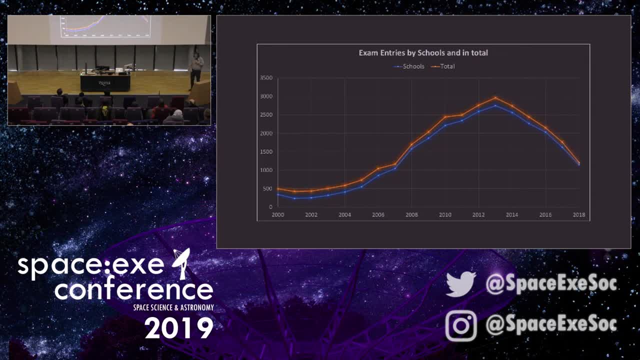 We need to be aware of what's happened since. That's what has happened since Now. I think there's a thesis there which says it's not a lack of enthusiasm for the kids to do this. I run GC astronomy after school. 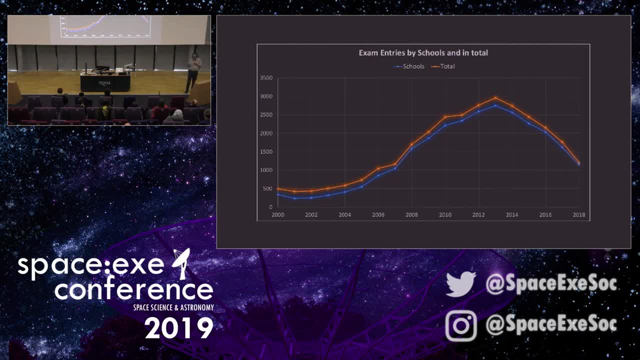 And I get kids turn up at the end of a school day for another two hours worth of study voluntarily. So let's just break that down a little. Is there a difference between boys and girls? Well, traditionally there are more boys that tend to do it than girls. 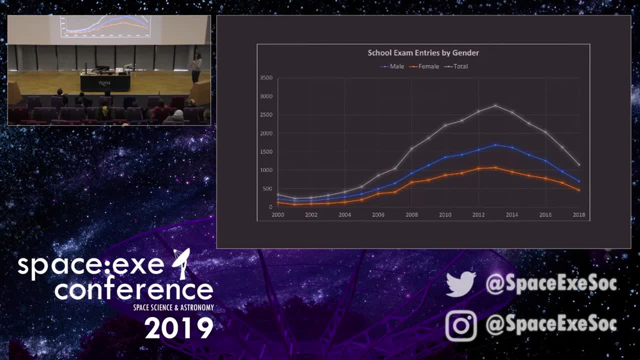 But it's not a minority interest for girls. What about the spread across the different institutions? Well, you can see that the total number, taking it is in blue, is about 1,000. So most of which are people at school. 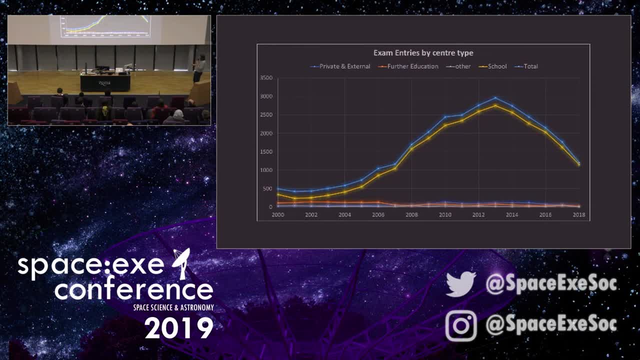 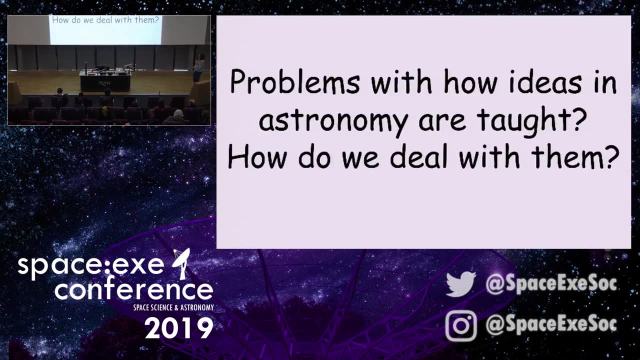 There are others in private or external entries or further education, But by and large, if you want to solve the next generation problem, you need to solve it in schools. So what are the problems with how astronomy is taught in school? Now I've got a bit of a bee in my bonnet about this. 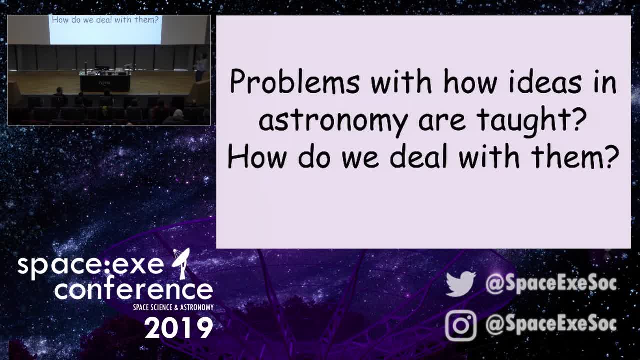 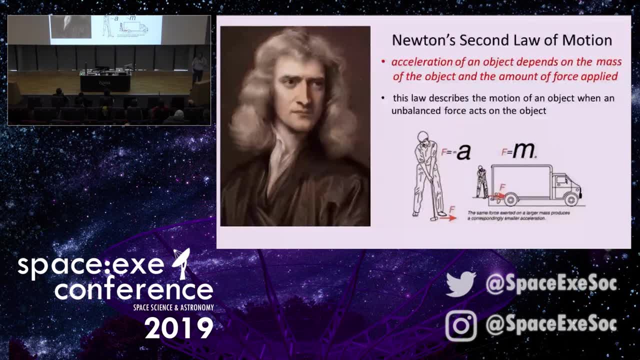 And I'm going to share it with you. I hope you're all right with this. First of all, we are encouraged. But why is this? Well, you know, I was in the secondary school and my teacher was teaching math when I was in high school. 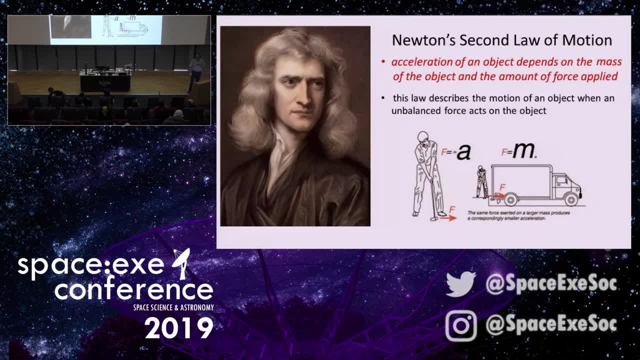 So my teacher was talking about how science and literature can make people feel alive, because they don't want to be raised in that little world. They don't want to be used as objects to keep them alive, And so my idea is to present important things. 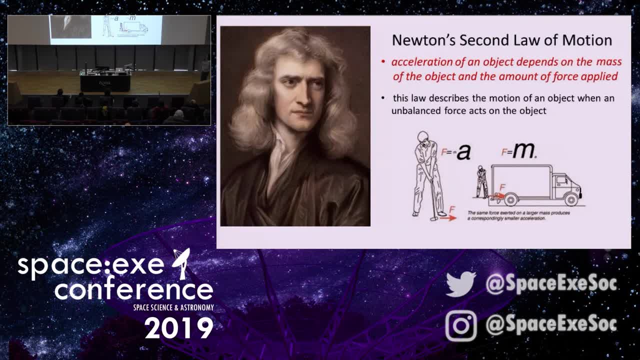 in a simplistic way for children, because they cannot understand this. Isaac Newton- and he talked quite correctly about the acceleration of an object- depends on the mass and the amount of force applied, which, as you get on, you realize that that is absolutely true, and every spacecraft that travels and everything else ties in with that law. My concern: 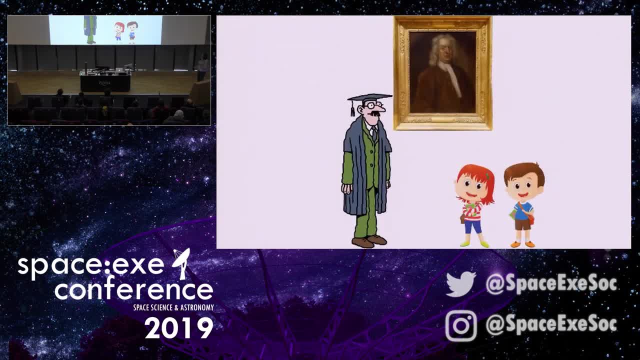 is the way that it's taught. So there's my little setup, says the teacher is saying Newton found that things require acceleration. sorry, they require a force to accelerate, but you don't need a force to maintain a constant speed. And so your pupils there are saying: hang on a minute. 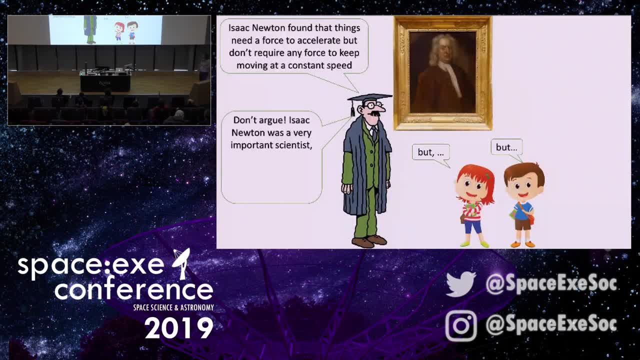 just a minute and the teacher will then say: don't argue. Isaac Newton was a very important scientist. I told you this lesson last lesson, the previous lesson. why don't you understand this, Not realizing that what the kids are thinking is this? 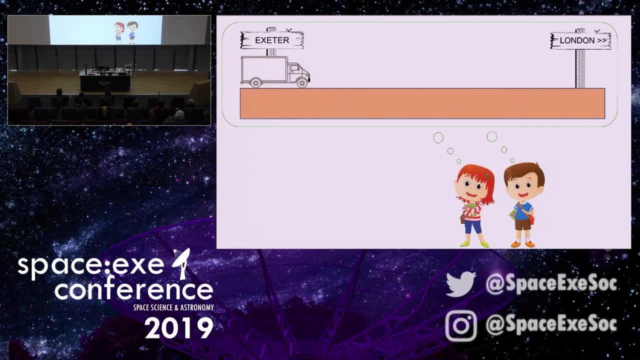 Well, here I am. I'm in Exeter and there's London. So, according to Newton, if I go up the M5 and head off to London, I only need petrol while I accelerate up to 70 mile an hour. Then I can coast all the way to London. 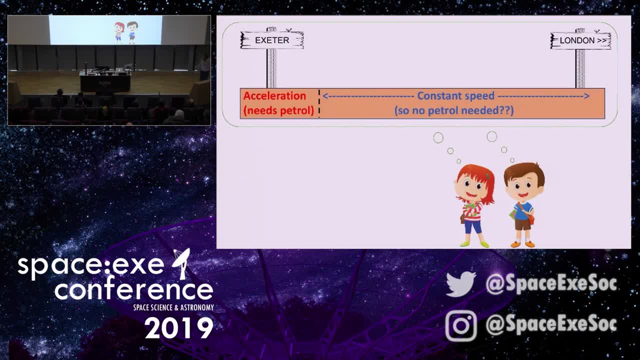 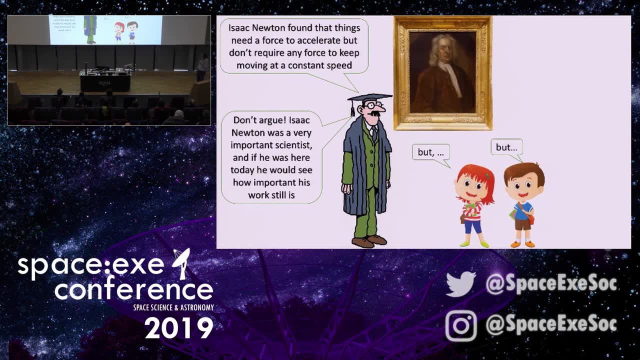 Now it's no good for kids who have got that internal message coming back and saying: but Isaac Newton, don't argue. Isaac Newton was a very important scientist And if he was here today he would see how important his work still is. Not realizing what the kids are whispering to one another is. 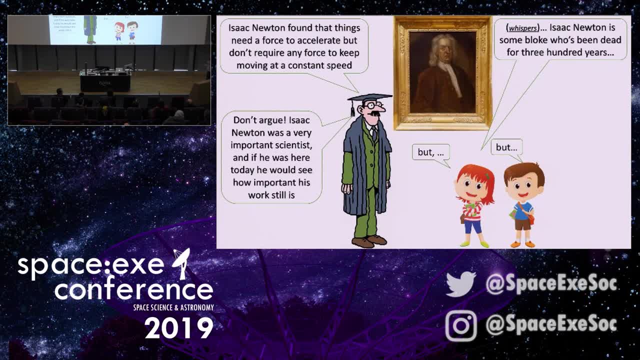 Isaac Newton was some bloke who's been dead for 300 years And, what's more, if he was here today, his car would probably keep running out of petrol. he'd be late for everything. If you want to take children forward, you have got to start where they are and move them forwards. 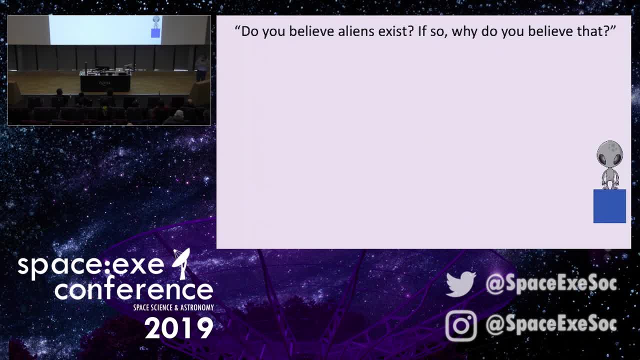 Okay, Oh, incidentally, I just slipped slide in I think. yes, I've got time for it. I slipped this one in. Some years ago I had gone with a group of teachers to NASA to get some teaching materials and brought it back. 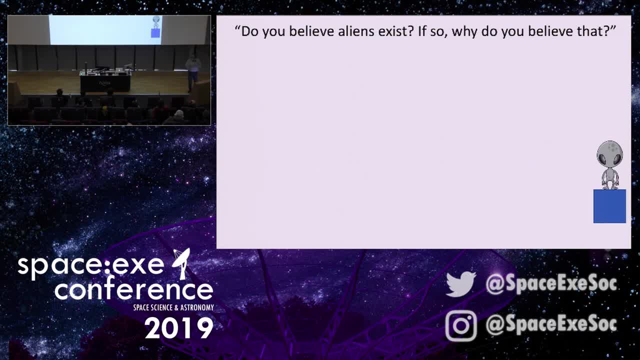 And one of the things they said was: it's a good idea to establish what the kids know already And we want to use multiple choice. but the trouble with multiple choice is if you ask somebody a question and the correct answer is answer C, everyone who knows it's C will score. 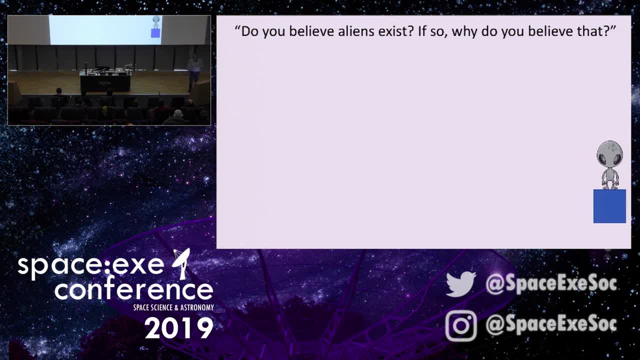 and everyone who guesses it's one of them and just randomly chooses C will get it right. So we tried to set this up where we asked for different concepts in different ways and just looked at the ones where the different questions over the same concept. 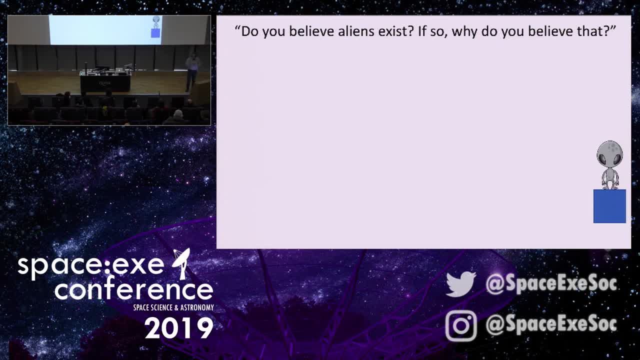 we looked to see which students really understand the concept and which one does. it appear to be random. It was interesting. They believe, yes, that aliens exist. Would anyone like to guess the answer to the follow up question? We had loads of different. 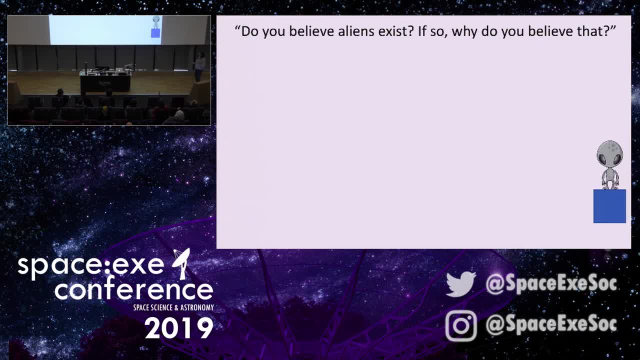 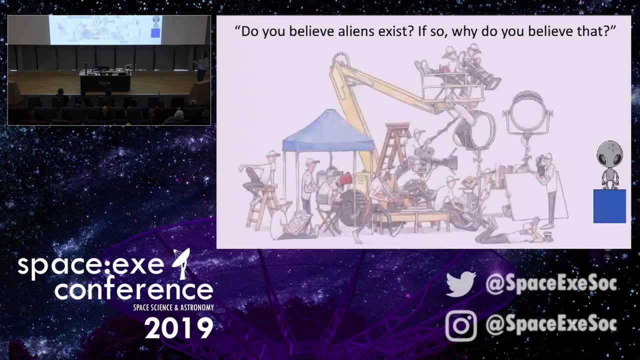 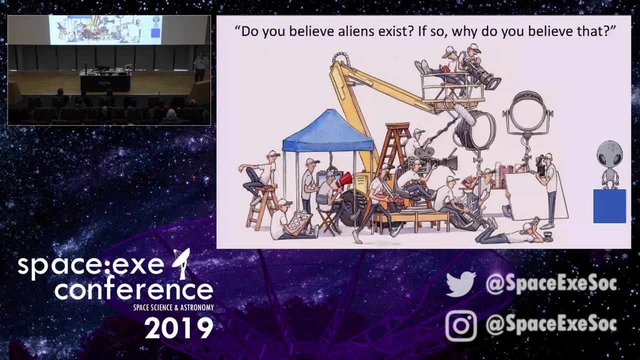 answers, But the most common one. anyone like to make a guess as to why young people believe that aliens exist? Well, there it is. Hollywood would not spend so much money on things that don't exist. Hollywood do spend a lot of money on films, Therefore they must exist. 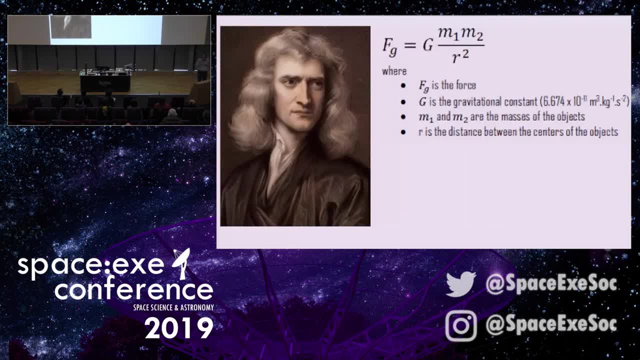 You're going to think that I'm picking on you. No, I'm not. His is such a fundamentally important thing. We got to make sure that children are taught it in a way that makes sense And it's not earth based. 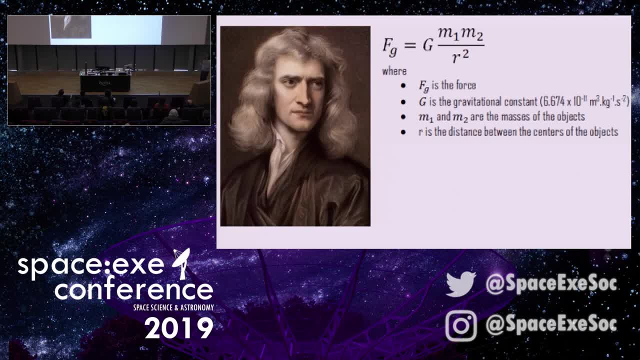 It's got to work on earth and everywhere else as well. So he came out with this universal formula. That's a formula that's used in every rocket or spacecraft that goes to any planet anywhere else. We've got to be able to deal with this, Unfortunately. to make it simple, 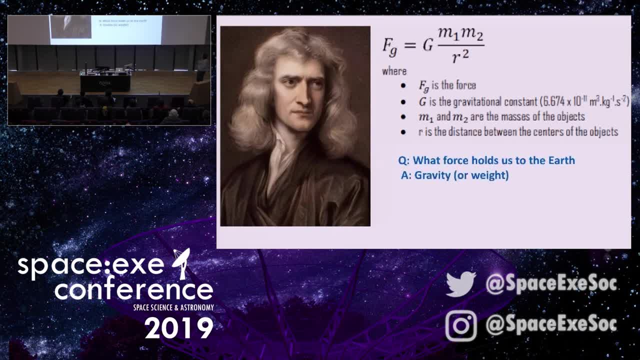 that's how children are normally taught What force holds us to the earth- Gravity or weight. It's a nice way to work. It's a nice way of introducing it. Later on we try and substitute that Weight is a force caused by gravity. 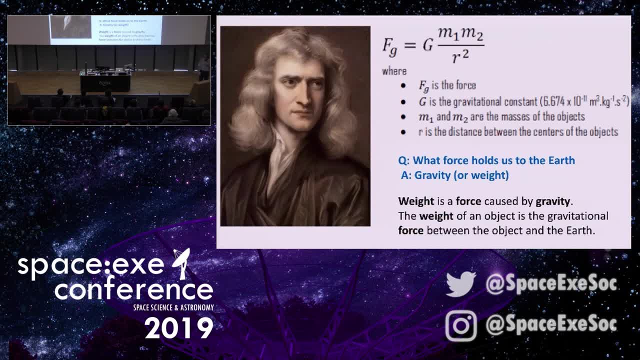 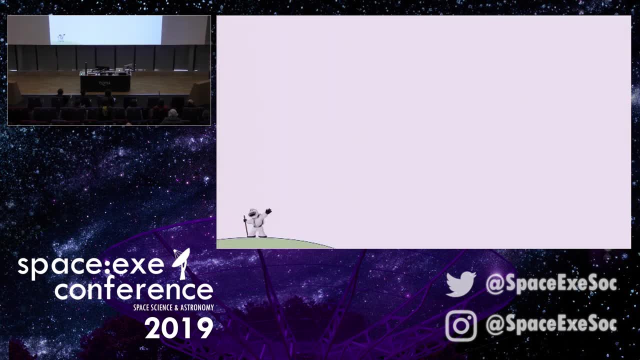 The weight of an object is a gravitational force between the object and the earth. I have to say I still don't think that's sufficient for getting the idea across, And my reason is for this To try and represent this. First of all, we ask children: what do you understand? What holds you to the surface? 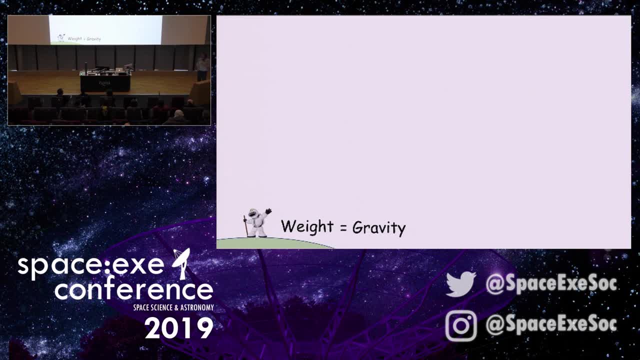 So what weight does? Oh, we've also learned that gravity is a force. We've also learned that's also gravity. Great, What have you got? What about this? What about spacemen out in space? What can you tell me about them? 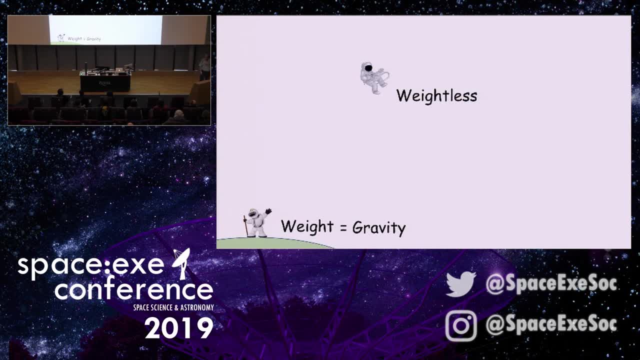 Oh, they're weightless. Unfortunately, they put two and two together and they will conclude that as well. Then you've got a real problem. Because if you then pursue it and say, OK, so what's the difference? Where does one change into the other? 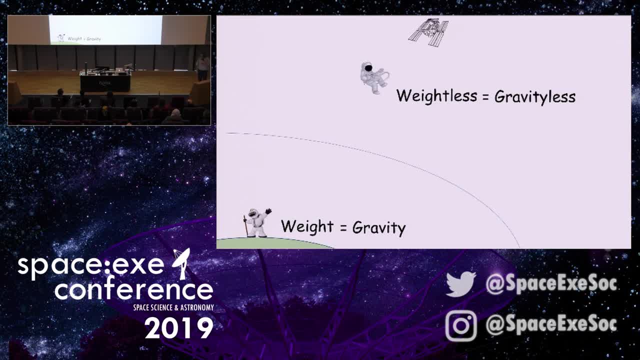 They say, is it when the air runs out? Seems to make sense. Airplanes up in the air running out of fuel or whatever will crash back down to ground, But stuff out in space. even the International Space Station floats out in space. 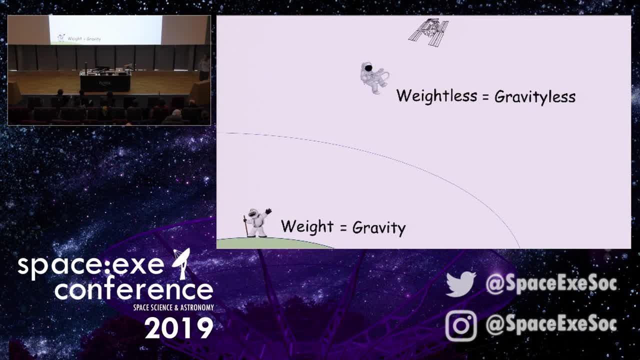 So, without being guided to what they're learning, they're going to come out with that. The interesting one is when you ask them: yeah, so what about that? What keeps the moon in orbit? And they'll come back with an answer. 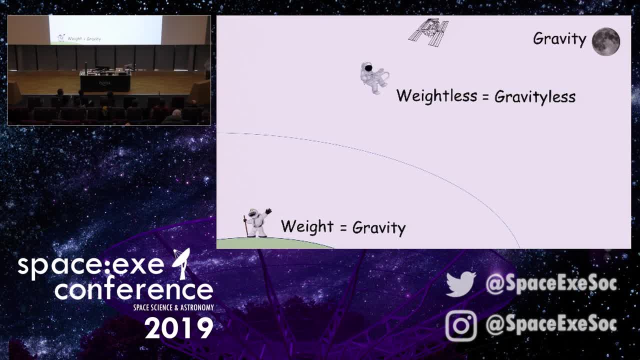 It's gravity. How does that work? How the hell does that work? We've got a gravity field. then no gravity, then gravity. Ah, the moon is big, The moon's big enough to have gravity, whereas the International Space Station. 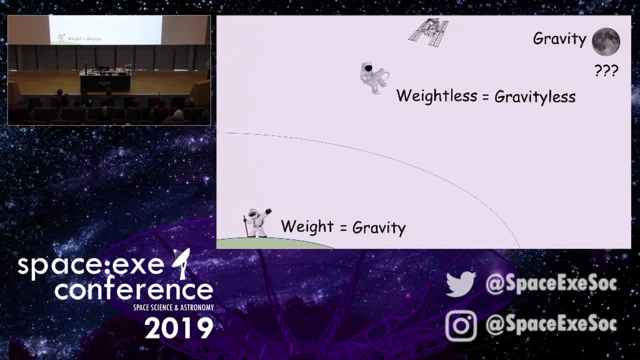 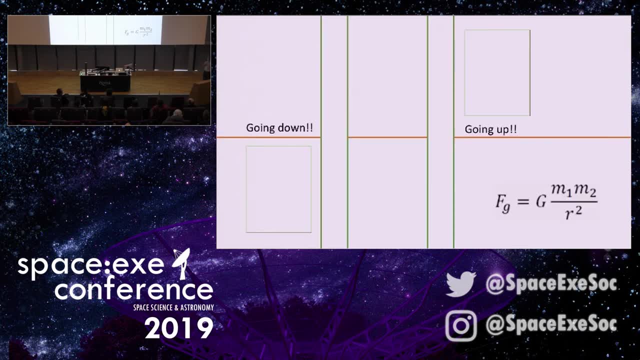 and spacemen don't. And it all comes back to this idea of making it simple in primary schools and saying gravity and weight are the same thing and they're not. Sorry, OK, Just to make it a bit quicker on this Going down, I'll run through this very quickly. You must have been in a lift If you believe that that is true and that's the full story, without anything else. you get in a lift, going down and your weight will actually get less. You go up and your weight will increase, Shooting through this rather quickly. 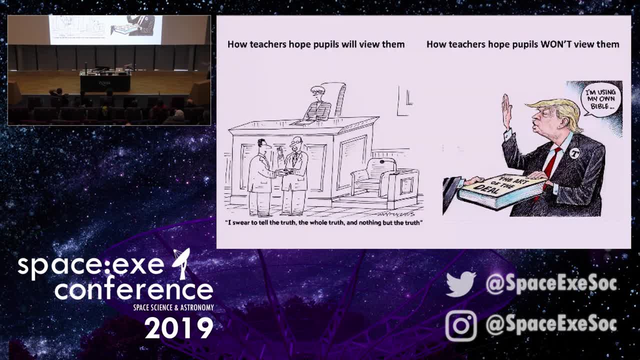 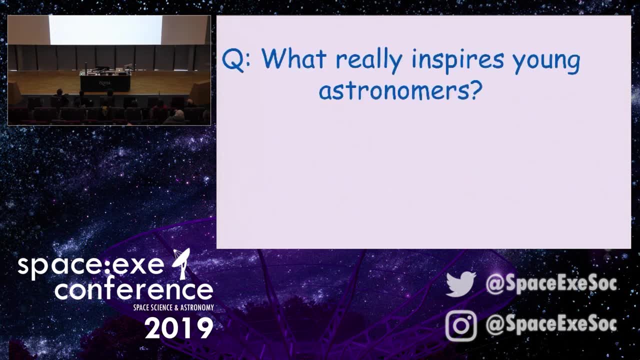 So we've got to be careful that we would like to be the ones on the left, but we want to make sure our kids don't think they're the one on the right. OK, let's just go through. So what really inspires young astronomers? 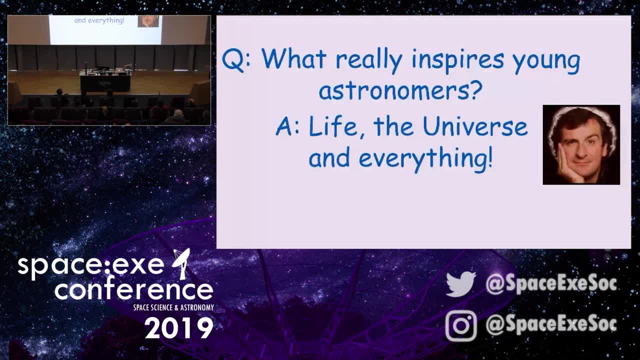 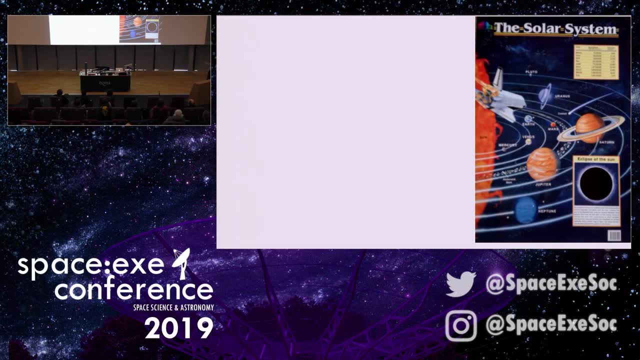 Life, the universe and everything. Thank you, Douglas Adams. And here I thought I'd just give you a couple of examples. First of all, if we show kids things like that, our problem is that gives the impression the Earth is very close. 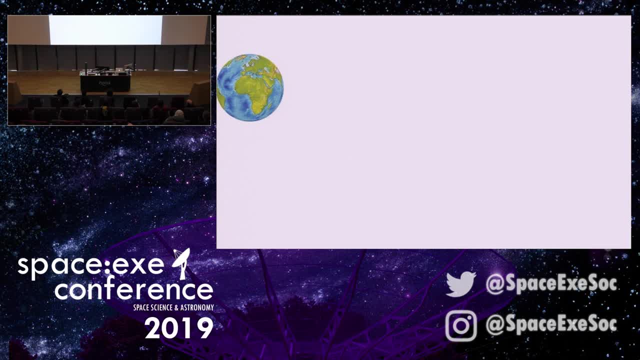 to the Sun. So there's the Earth. if you pose a question to them, saying you're not used to using rockets and light may only take eight minutes, but suppose we use something that you're used to, like a train. Suppose we were to send a train. 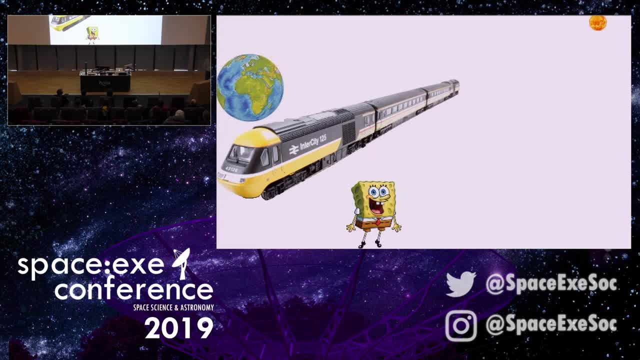 to the Sun. How long would it take? Intercity 125.. Unstopping. How long does it take? You ask most people and they say: well, I know it's not going to take eight minutes, it's going to take weeks, probably months. 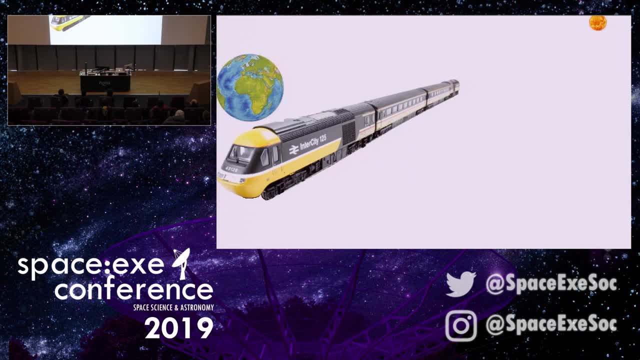 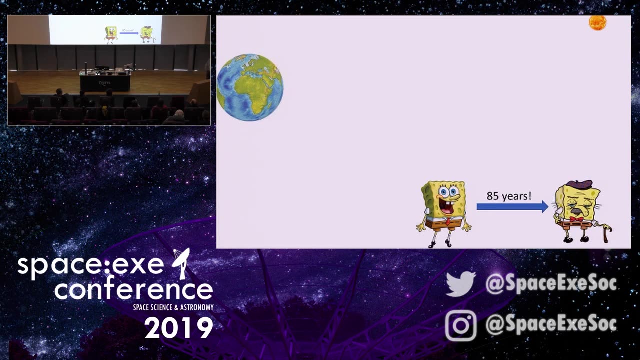 to get there, assuming you were to go without stopping. The interesting thing is The answer is 85 years. Kids need to get their answer right. The Sun might be close, but that doesn't mean it's really close. It's relatively speaking close. 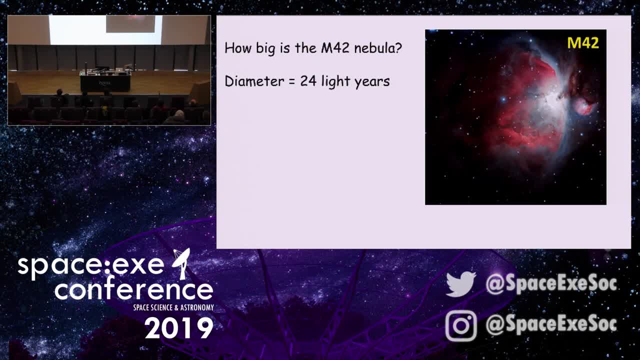 It's still 85 years away on a train. What about M42?? We saw that one earlier. Diameter: 24 light years, But that doesn't mean much. Kids don't quite understand what that is. So what's understandable units? 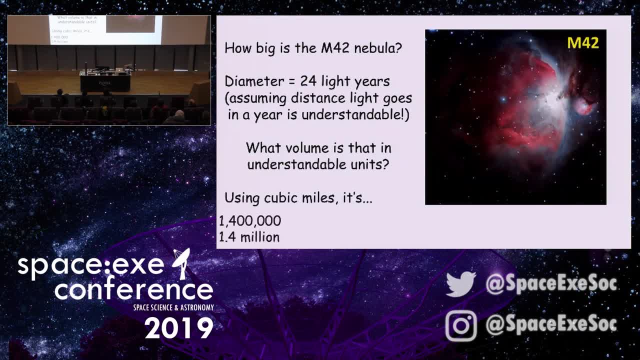 This is what kids are fascinated by. You put it in cubic miles. Anyone know what that's going to come out to be: It's 1.4 million million, million, million, million, million, million cubic miles. The universe is a big place out there.